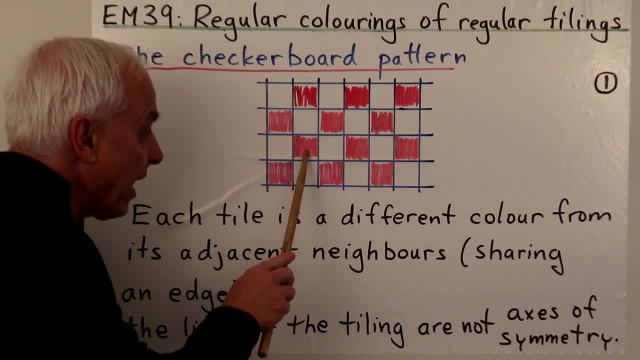 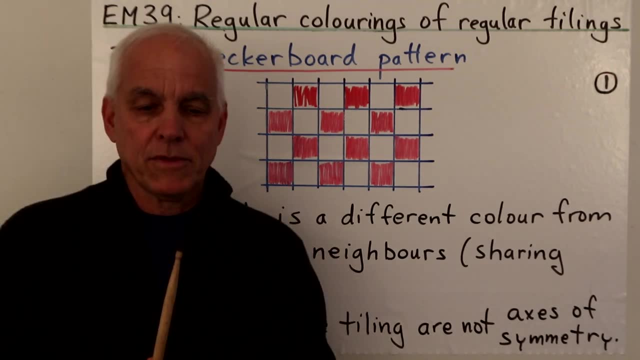 In this white as an edge, all a different color. So this red tile, its adjacent neighbors, are this one, this one, this one and this one, And they're all a different color. So an interesting question that I've gotten you to think about. 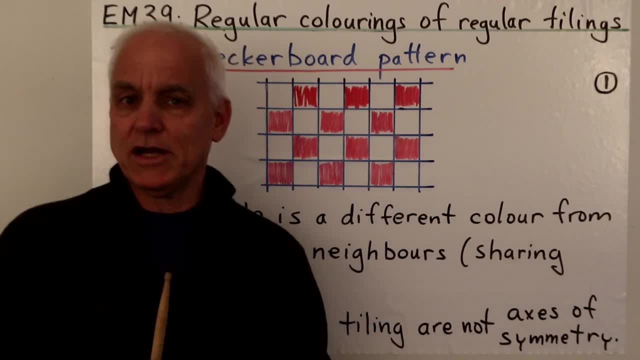 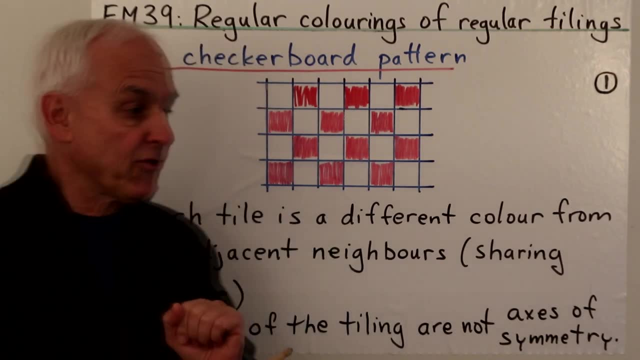 hopefully, is across. what kind of symmetries does a configuration like this have? And we're especially interested in mirror or reflection symmetries. Now, it turns out that once we color the checkerboard, Nowit turns out that once we color the checkerboard, 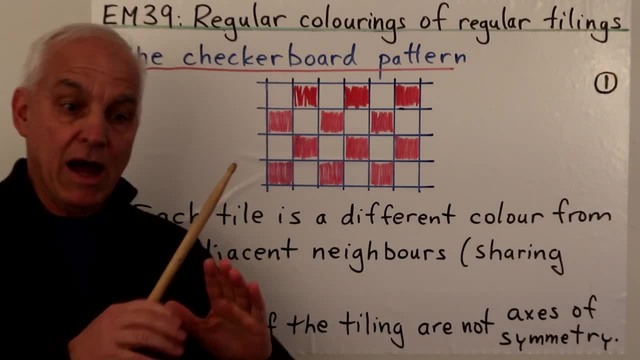 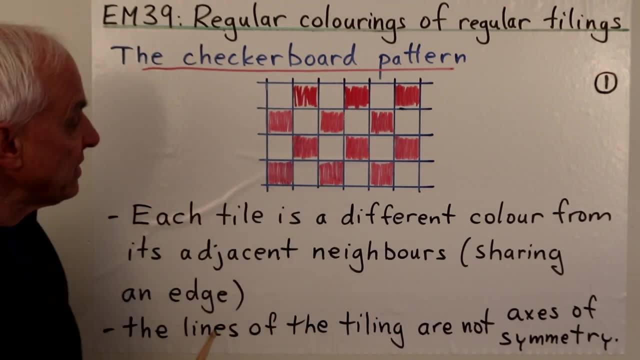 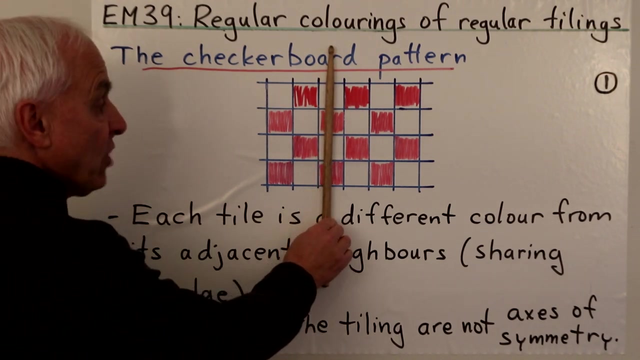 the number of symmetries that we had with the uncolored tiling reduces, And let's have a look why. So what kind of lines of symmetry does this pattern have? Well, this vertical line, for example, is still an axis of symmetry. 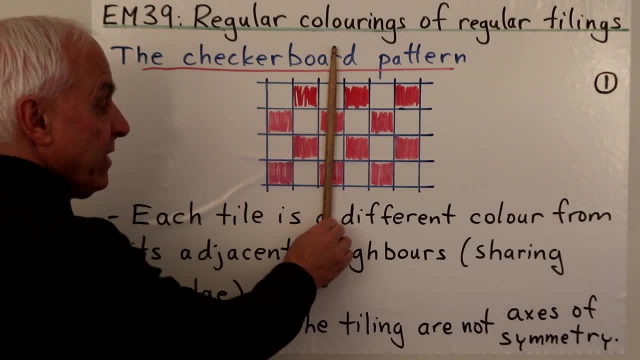 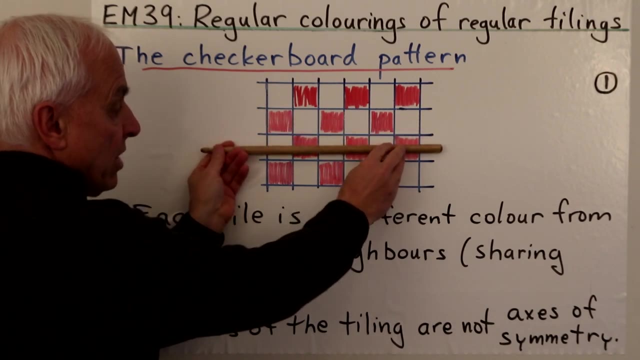 The whole pattern is symmetric when you reflect in that. So this tile here on the left-hand side is balanced by this right tile right here. Similarly, of course, a horizontal line that goes through the middle of these tiles will also be a line of symmetry. 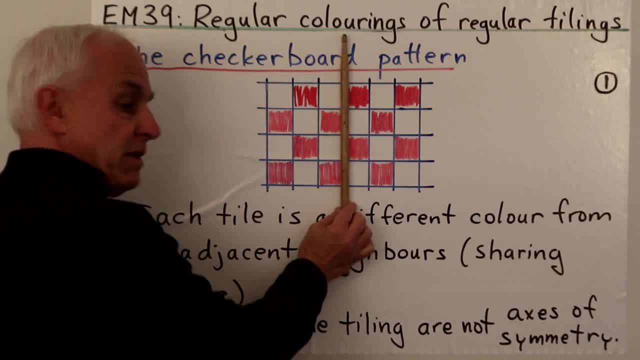 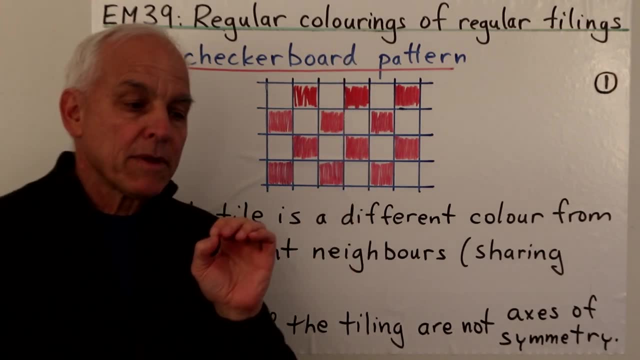 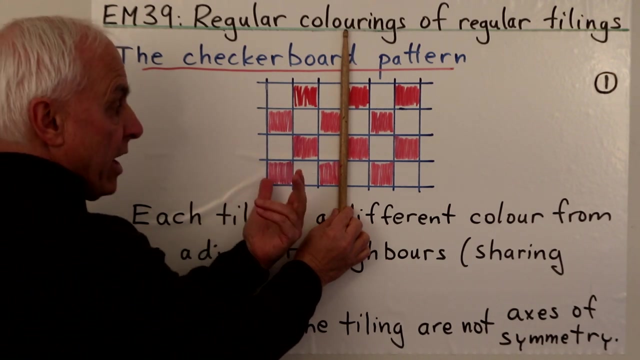 But interestingly, the other kinds of lines of symmetry of the uncolored pattern, namely the lines of the pattern themselves, are no longer axes of symmetry of this colored pattern. So, for example, if you look at this line here, if you reflect in this line, 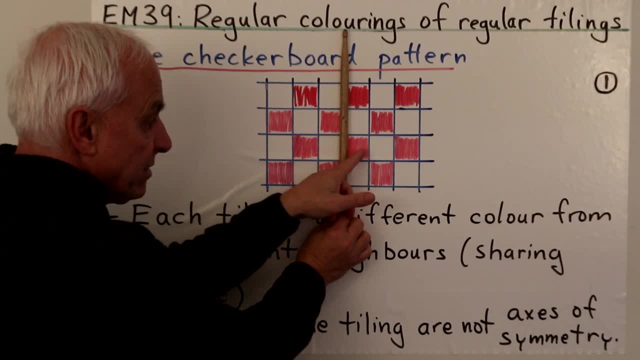 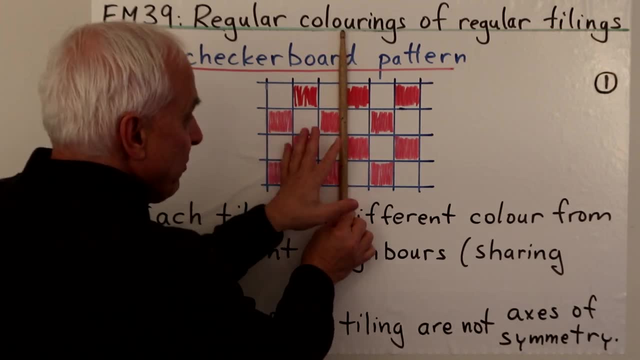 there's no longer a symmetry. So there's a red tile on that side, There's a white tile on that side. They're different colors, so it's different. okay, So the symmetry is broken. This is no longer an axis of symmetry. 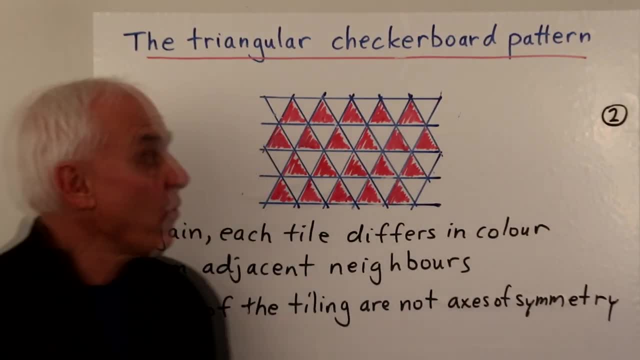 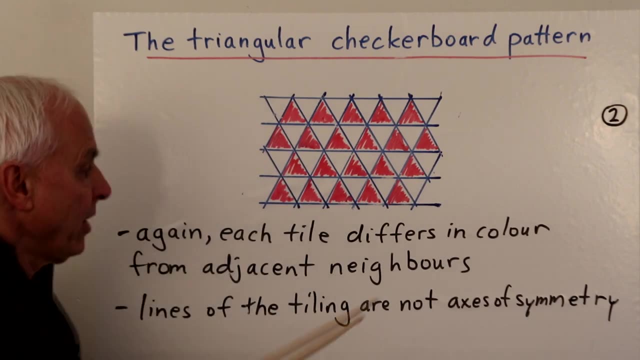 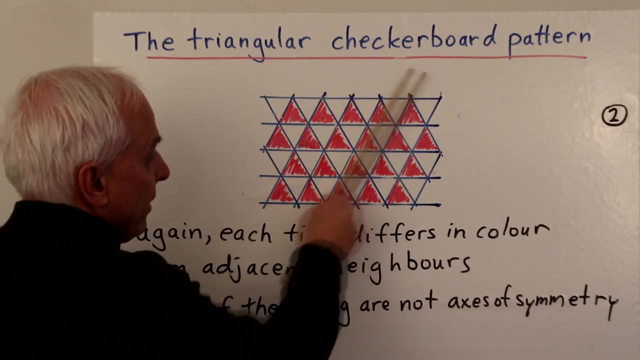 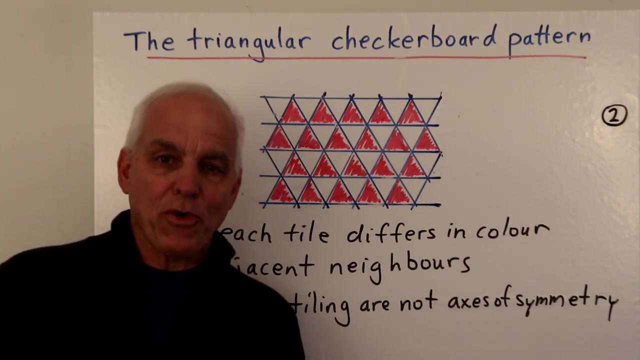 So here now is the analogous picture for the regular triangular tiling, made up of equilateral triangles, And it's created by having three families of parallel, equally spaced lines: That one and also this family. okay, And now we're also coloring it in a checkerboard kind of fashion. 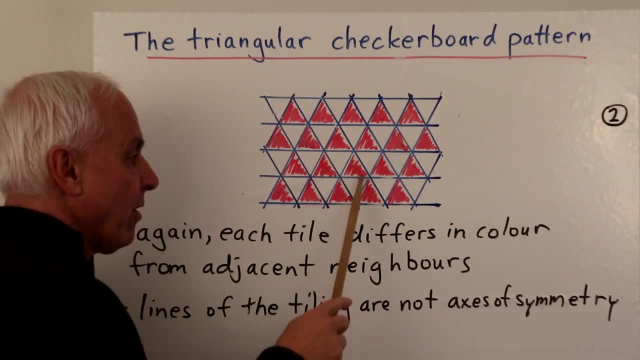 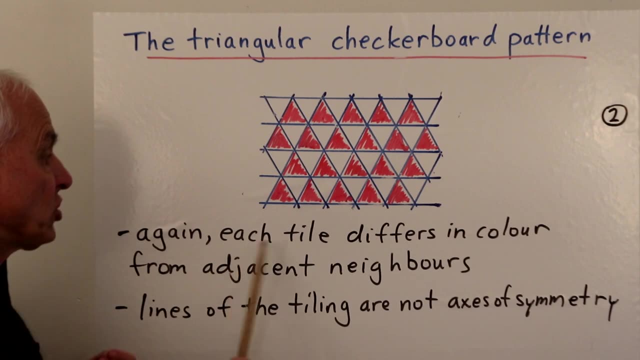 sort of alternating white red, white red in all directions, And it has the same property that the checkerboard pattern did that we just looked at. Namely, each tile say that one there differs in color from its directly adjacent neighbors. 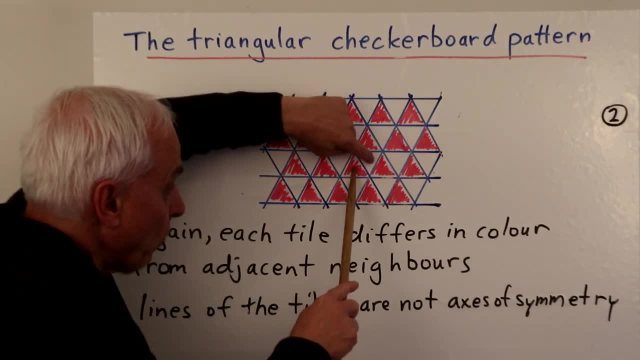 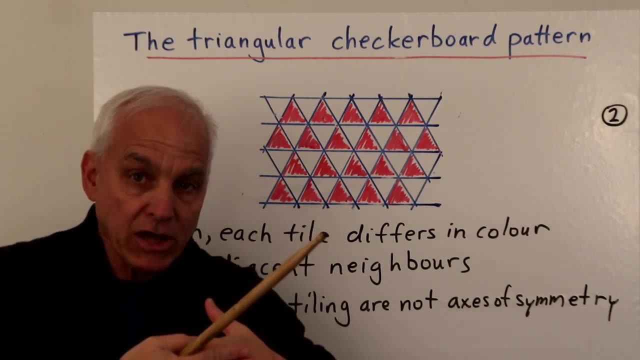 So this tile here has directly adjacent neighbors: that white one, that white one and that white one. So whenever we cross from one tile to a neighbor, through an edge, through a common edge, then the color changes. So that's actually quite useful, right. 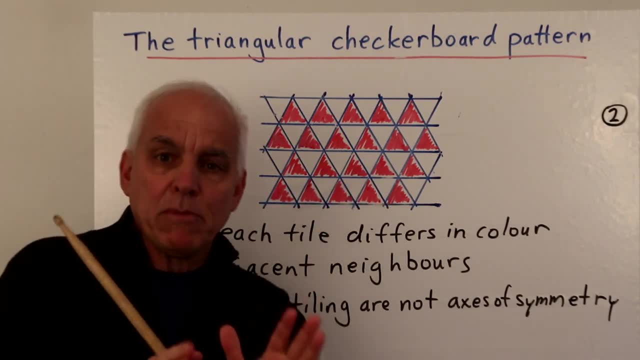 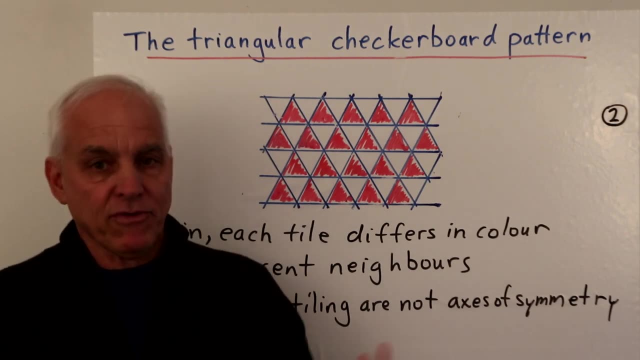 In demarking the boundaries of something a little bit more prominently visually, Because having colors is an aid in separating things. That's why maps of the world often have different colors representing different countries. It makes it clearer. you know what the various countries actually are. 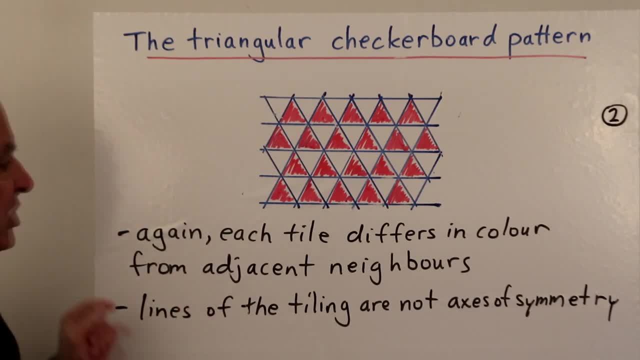 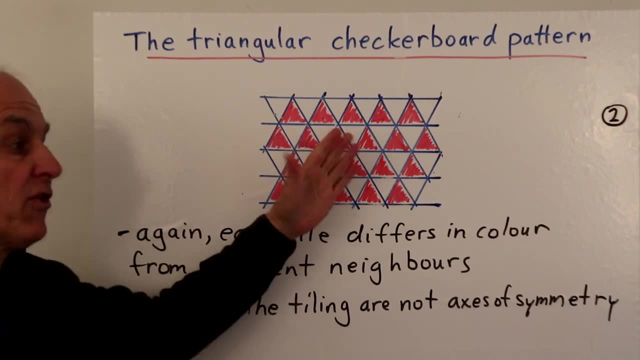 So we're just looking at it visually And we have the same observation as we did in the previous case: that the actual lines of the tiling are no longer axes of symmetry of this colored pattern. So, for example that line, there is no longer an axis of symmetry. 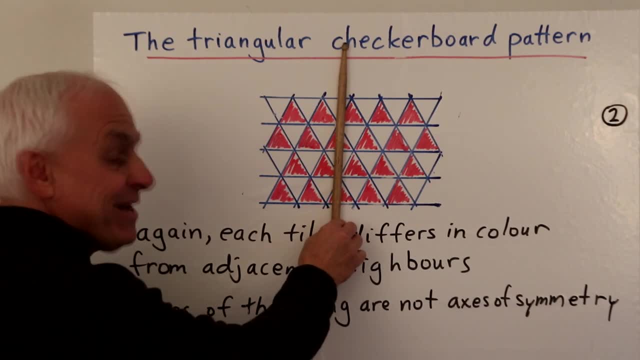 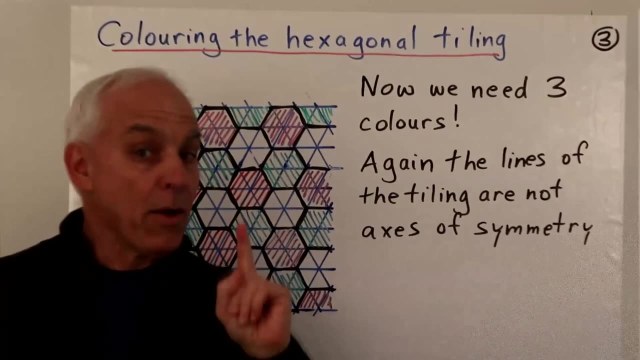 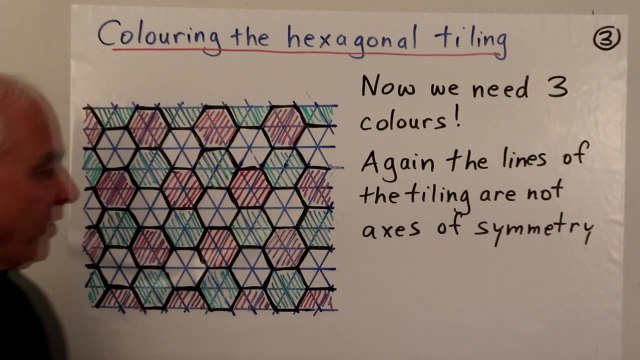 However, this kind of line is still an axis of symmetry, as is this one, as is this one. So now we come to the hexagonal tiling, our third regular tiling, And here things are a little bit different. So here's the tiling. 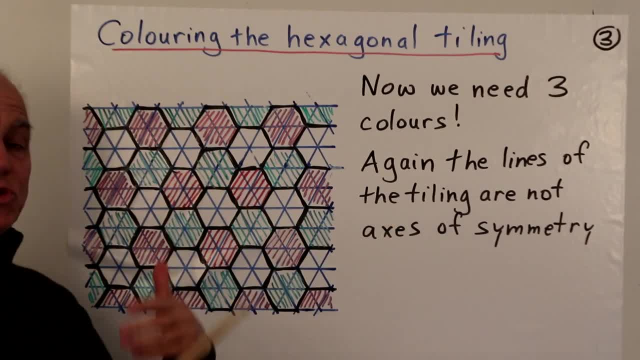 It's got a lot of these regular hexagons and it's created by being superimposed on an underlying triangular pattern. And here we see that we've colored the pattern, but we've used three colors: White, red and green. 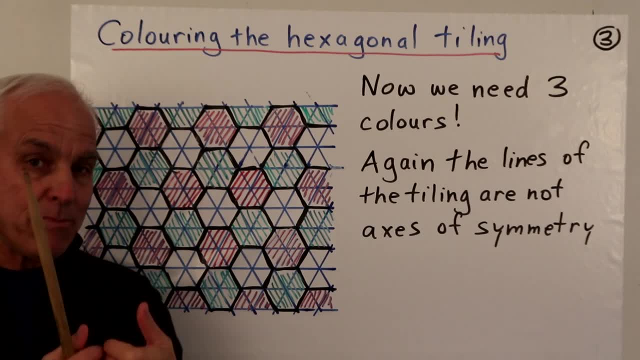 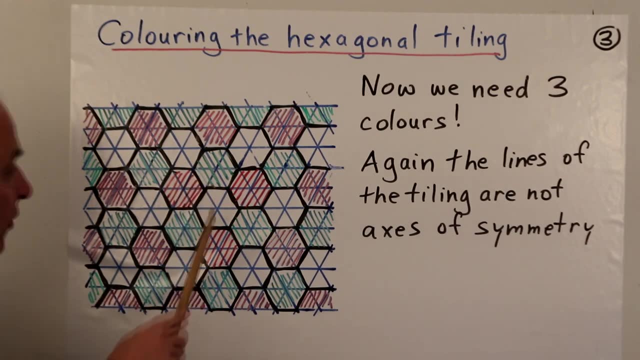 And we need these three colors if we want this same property: that across every adjacent edge we're changing color. So going from here to here, we're crossing that edge. we're going from white to red. Going from here to here, we're crossing this edge. we're going from red to green. 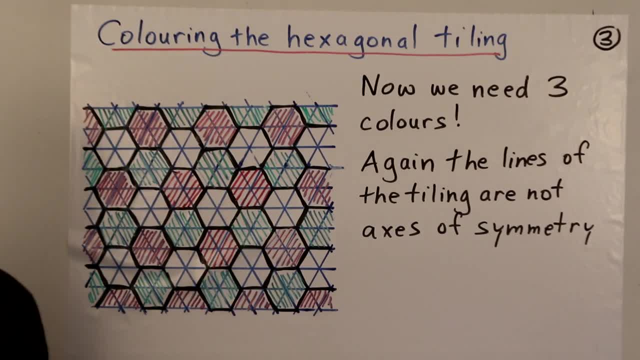 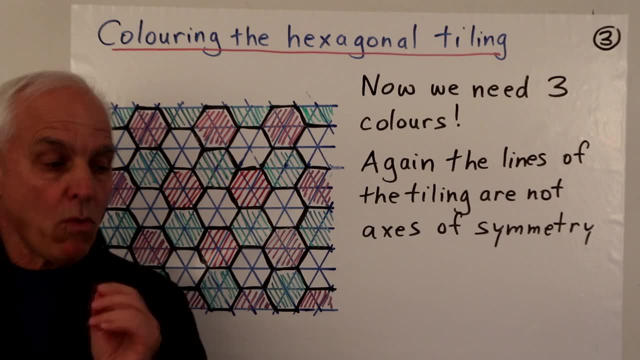 Going from here to here. we're crossing this edge and we're going from green to white. So what is it that makes this particular pattern sort of different from the other two? Well, one way of understanding that is by looking at what's happening at a vertex. 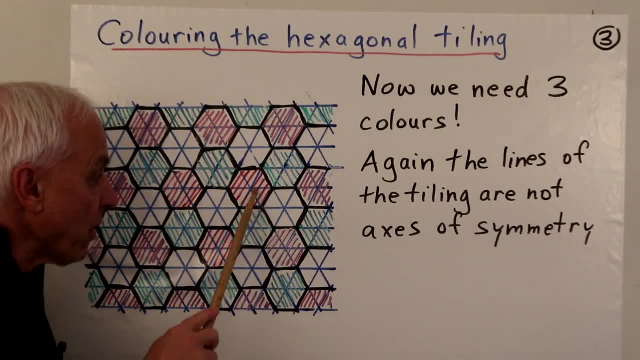 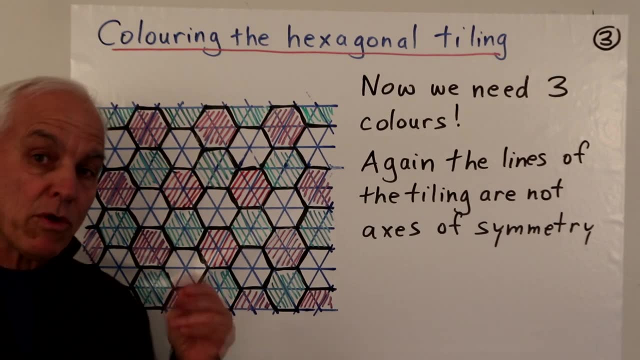 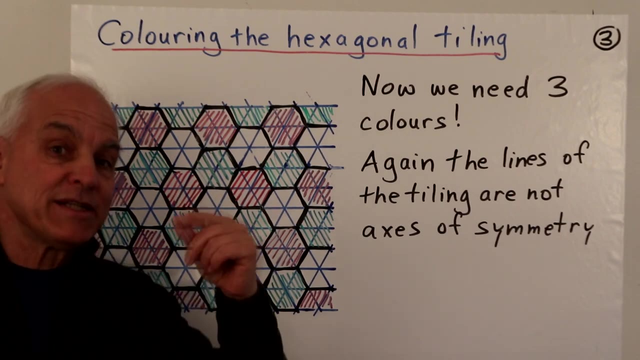 Look at that vertex. there, At that vertex, there are three tiles that are meeting, Three tiles that are meeting. In the case of the square, there were four tiles that met at a corner And in the case of the equilateral triangle tiling, there were six that met at a corner. 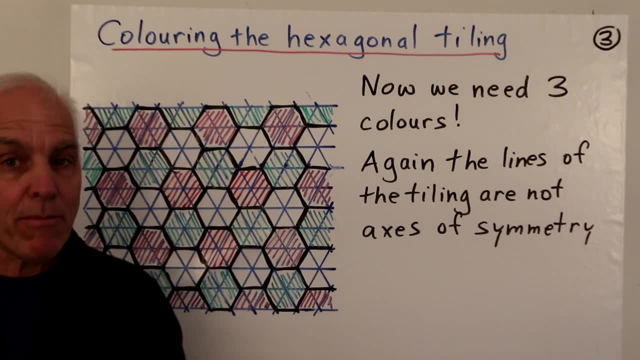 Now, four and six are even numbers And that means that as we go around one of those vertices- say, with four we can go white red and green Red, white red, And that's consistent. When we get back we're still alternating. 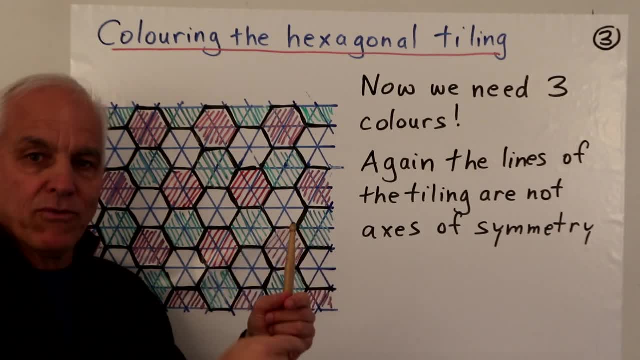 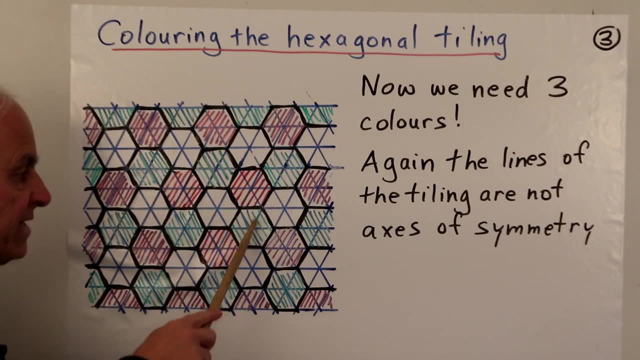 And the same. when we have six, We go white red, white red, white red, And then we're back to the white. But we can't do that with three, So we start here: white red. This next one can't be white and it can't be red. 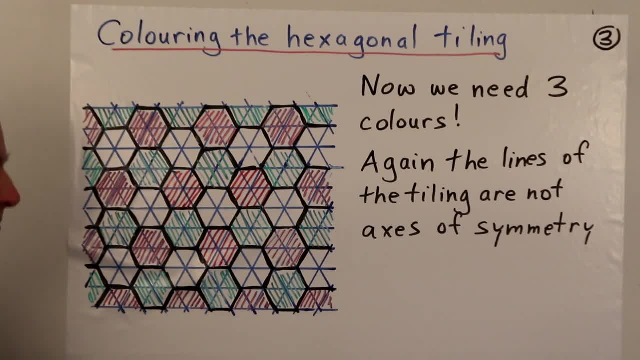 So it's got to be something different. That's an explanation, Okay, but otherwise the remarks that we've made before are sort of still holding up. The symmetries of this colored pattern are now reduced, And what do they kind of look like? 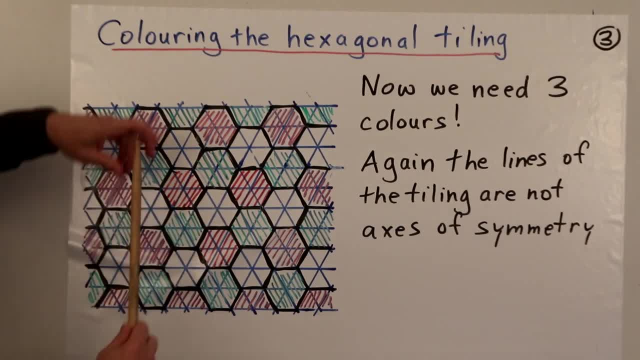 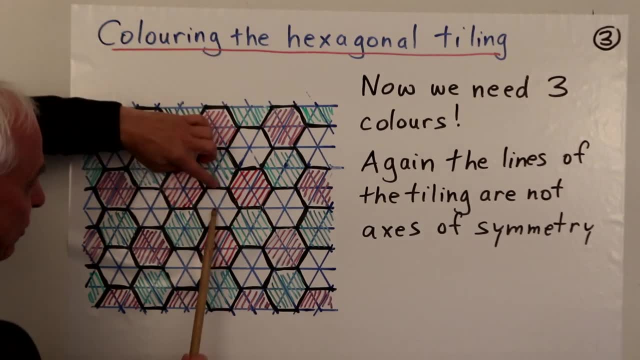 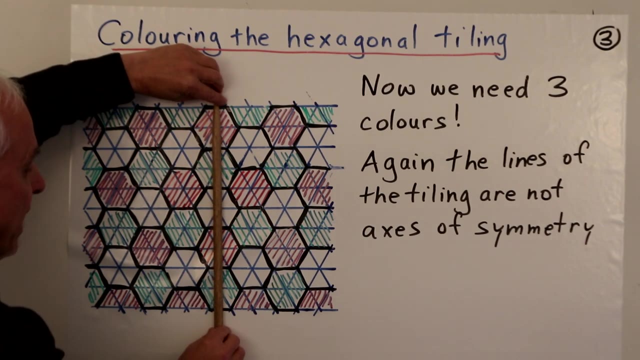 Well, if we take, say, a tile, say that one there for example, and we look at the axes of symmetry that are like this: so this axis of symmetry that goes through sort of the midpoints of opposite sides, if you have a look you'll, I think, agree that that's an actual axis of symmetry. 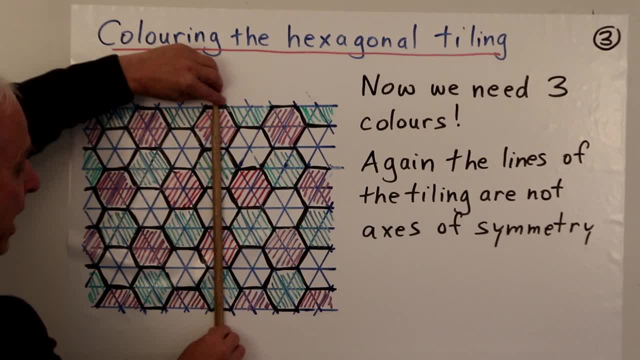 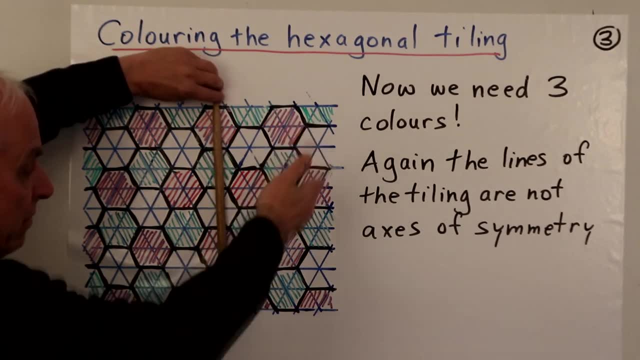 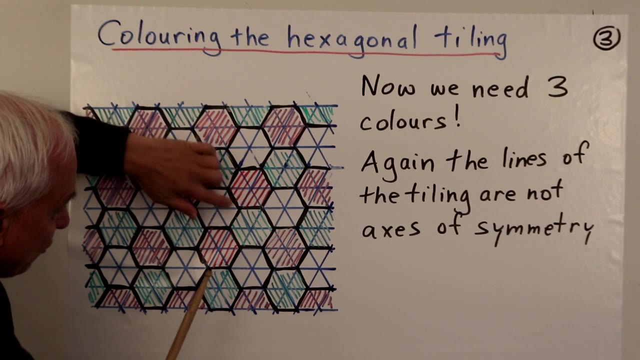 of the entire configuration And notice that that axis of symmetry does not actually coincide with any one of the underlying blue lines of the triangular tiling. However, if we look at another line of symmetry of this basic hexagon here, namely this one here: 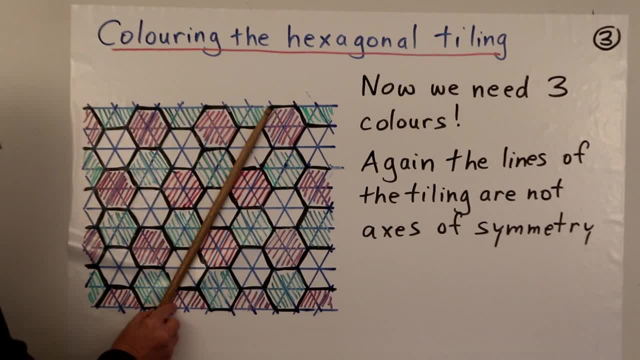 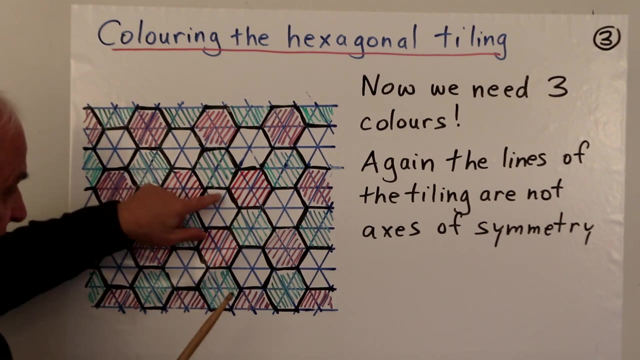 this is no longer an axis of symmetry of the entire thing, because you know there's a red one here and there's a green one on the other side, So it's not symmetrical color-wise. So instead of having these six axes of symmetry, say, centered at that point there, 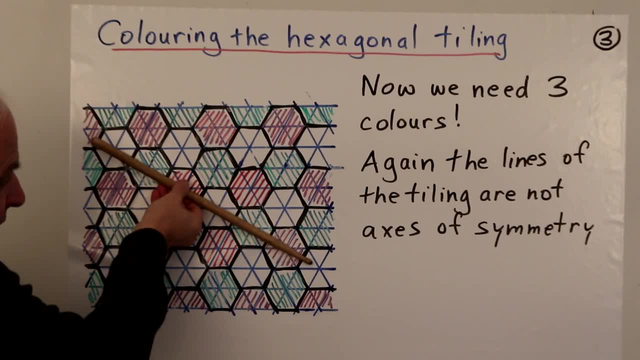 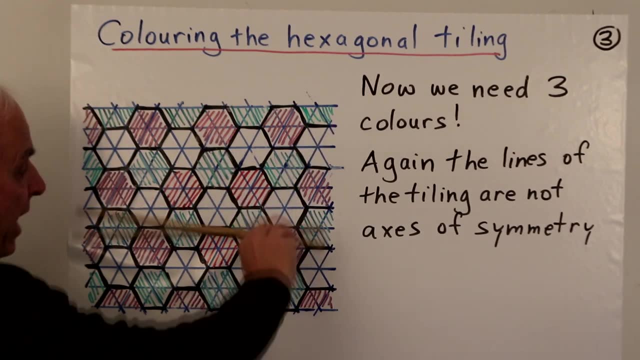 we actually only have three: This one, this one and this one, And in particular, the actual blue lines which are underlying things are no longer axes of symmetry. That's not an axis of symmetry. That's not an axis of symmetry, etc. 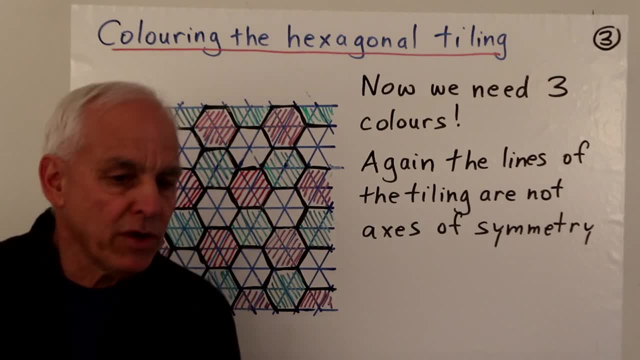 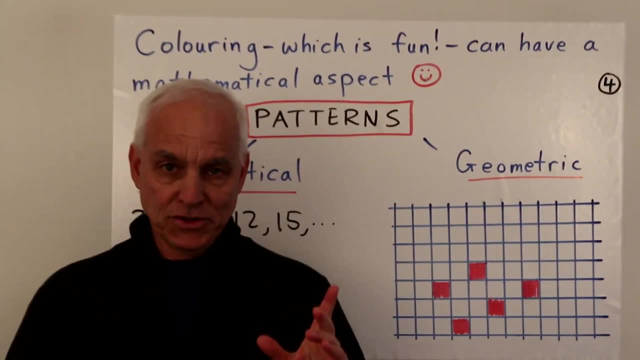 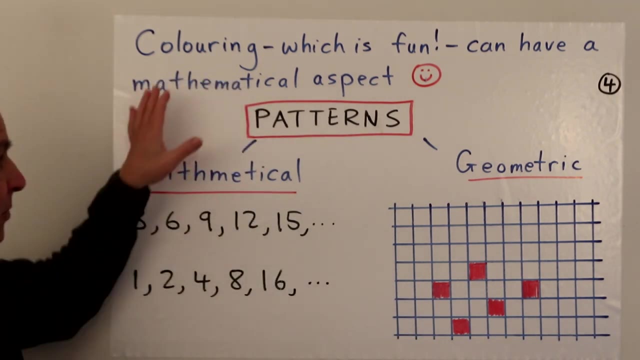 So quite interesting. This hexagonal pattern is a little bit richer, a little bit more complicated than the square and the equilateral triangle tilings Alright. so those checkerboard kind of patterns are sort of a starting point, but there's actually a wide variety of extensions to this. 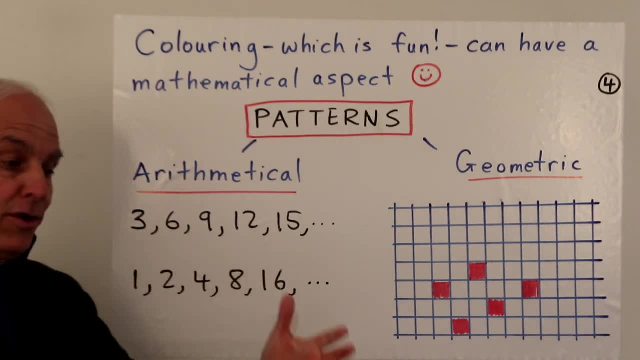 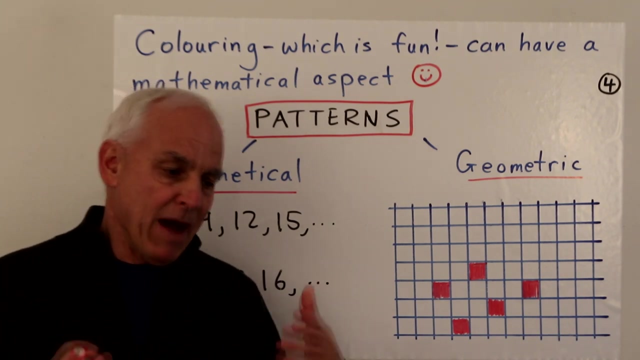 all centering around coloring and trying to get regular patterns in a geometrical context, starting with one of these three regular tilings. So the idea of the notion of a pattern is very important in mathematics, Very, very important. Mathematics is, to a large extent, the study of patterns. 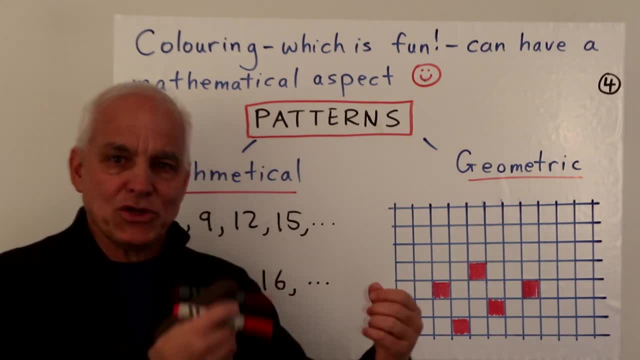 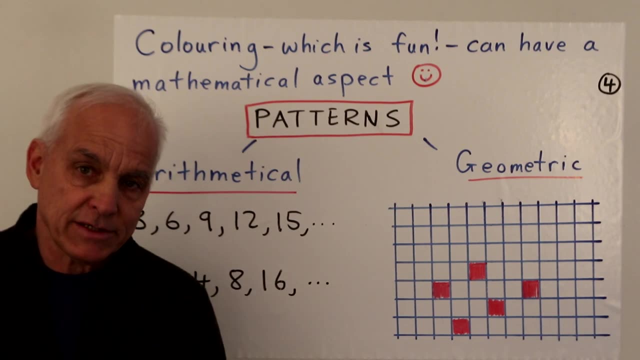 Identifying patterns, studying them, figuring out what's going on, And for most students, they'll be familiar with that in an arithmetical context, which is the most familiar one, For example, you may have a sequence of numbers. 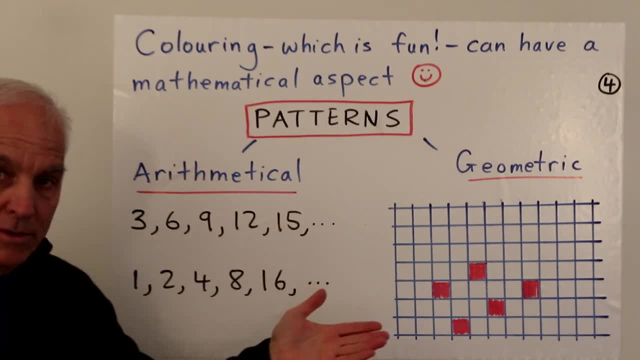 Three, six, nine, twelve, fifteen. What's the pattern? Well, hopefully we can tell. This is not such a hard one. These are the multiples of three, So the next one should be eighteen, and the one after is twenty-one, and so on. 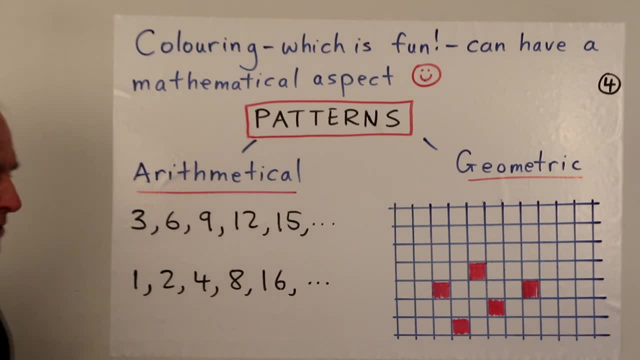 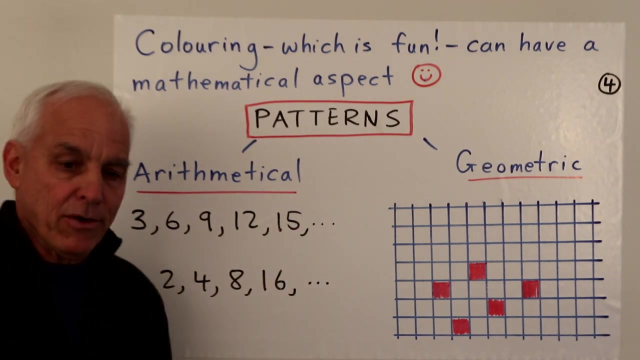 Here: one, two, four, eight, sixteen. It's another pattern. that's reasonably easy. Each one is just twice the previous, So these are powers of two. The next one should be two times sixteen, which is thirty-two. And of course there are hundreds of interesting patterns in mathematics. 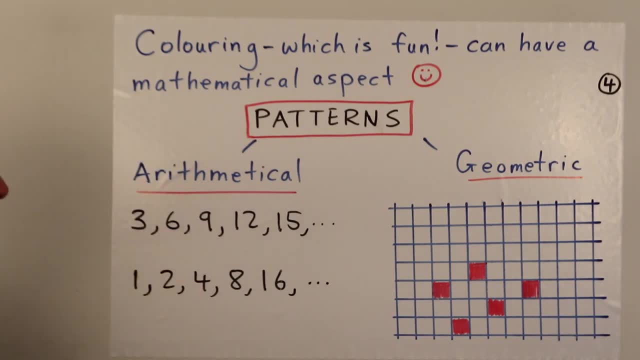 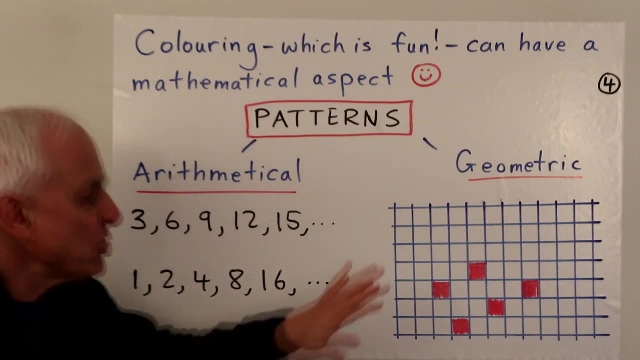 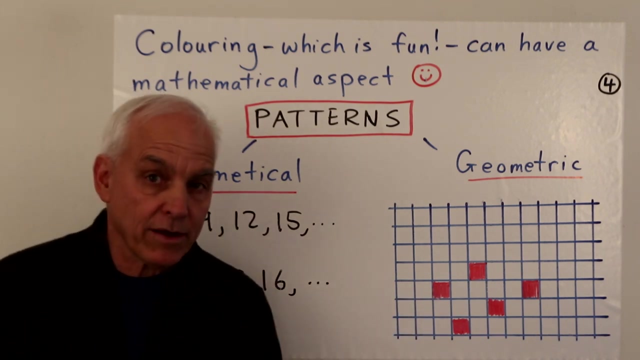 and some of them are a lot more complicated arithmetically, But what we're looking at today is a geometrical kind of analogue to this, which is much less investigated than this arithmetical side and is arguably just as rich and interesting. 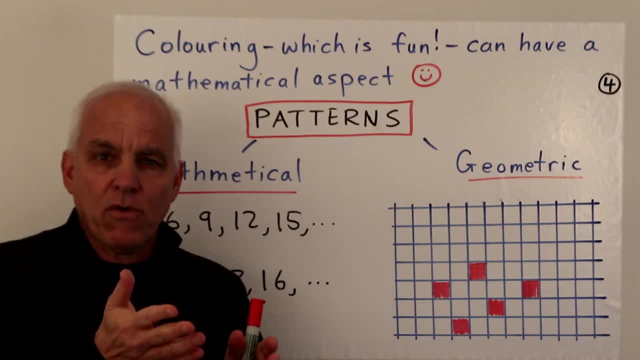 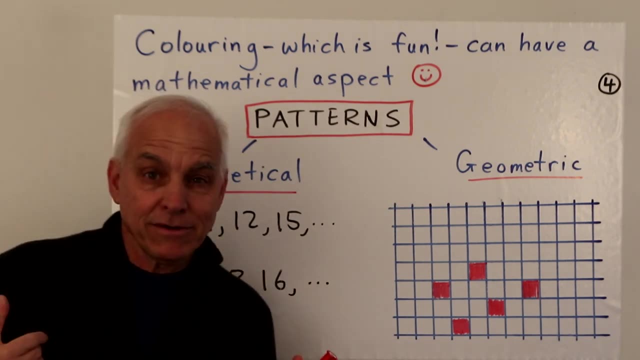 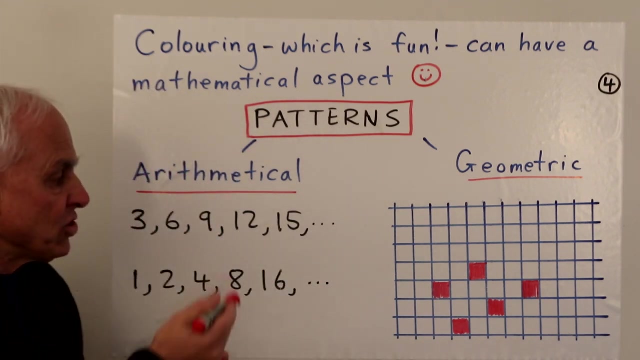 And it provides a great entry point for certain kinds of young people who are more visually oriented, maybe less arithmetically oriented. they may be artistic, they may have design interests, they might just enjoy the physical aspect of colouring. So you can attract them to mathematics by balancing this arithmetical stuff. 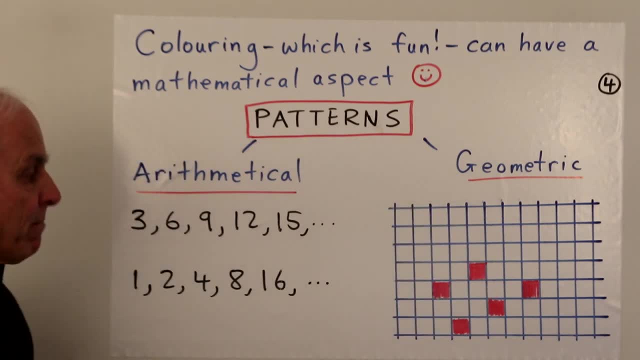 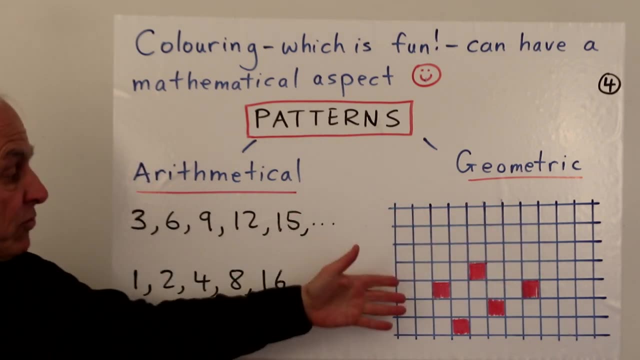 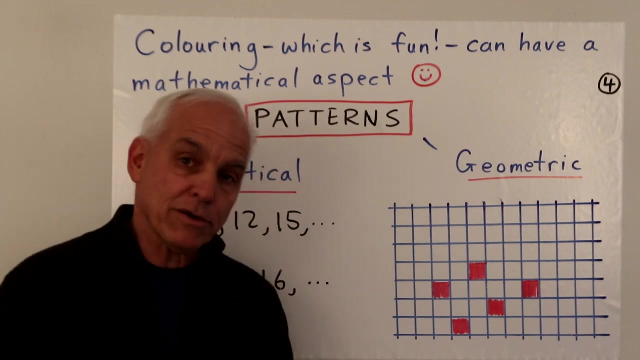 with some geometrical stuff. That's sort of the main message today. So let's have a look at this starting point. We're starting with the regular tiling, the simplest one, the checkerboard, the piece of graph paper, and we have, well, five squares that are coloured. 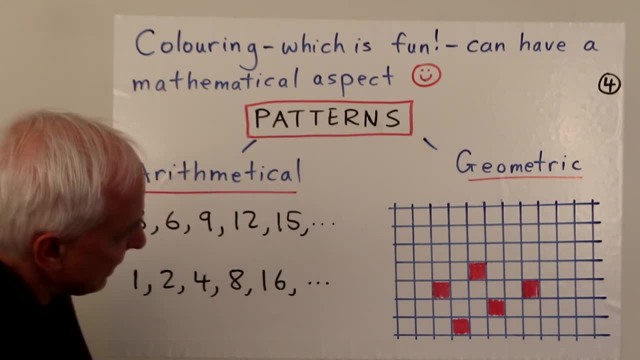 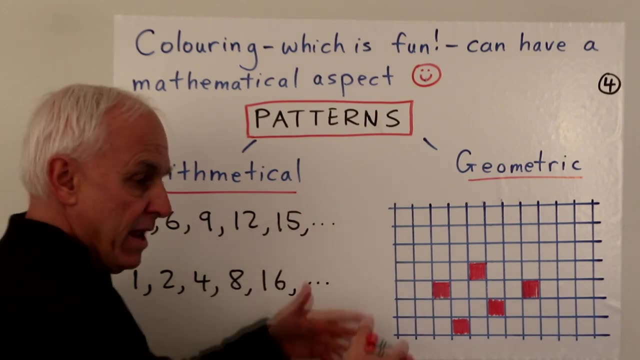 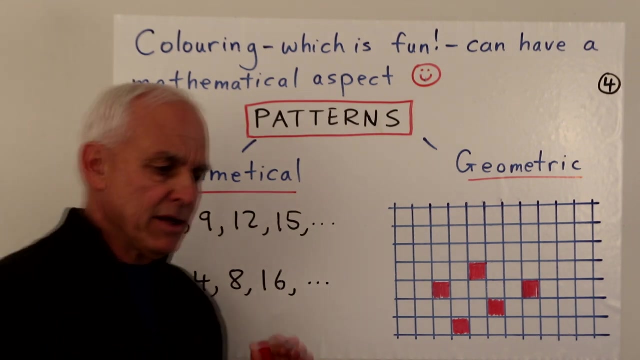 And you look at them, you see there's kind of some pleasing regularity there, and so an actual question might be: can we extend this? Can we extend this pattern to make a truly regular pattern in some way? Well, it turns out that that's not entirely a clear question. 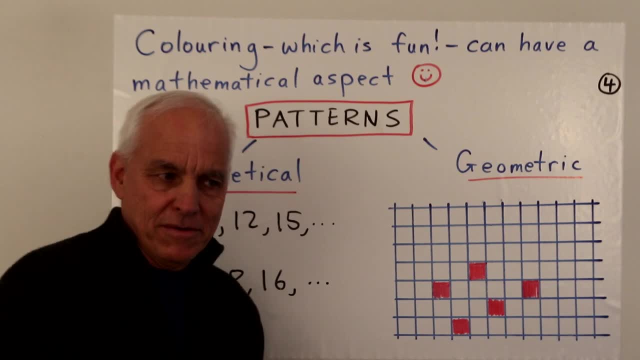 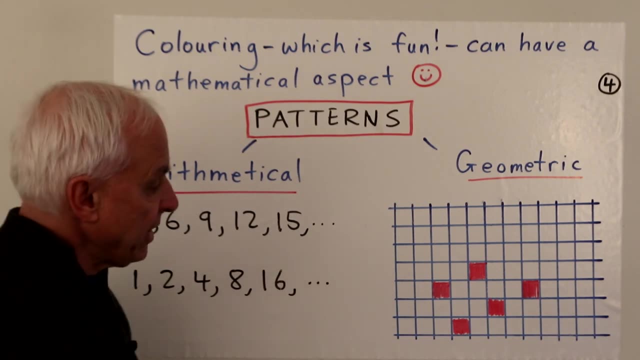 So there might be lots of different ways of doing that kind of thing: extending some given pattern to a bigger pattern, which is kind of regular. But in this case I think you'll agree that there's kind of an obvious thing, and so I'm going to do a little bit of it. 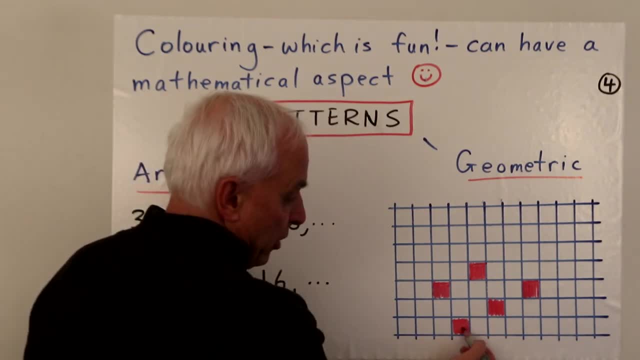 So I'm going to notice that, say, to go from here to here, we're going over two and up one and over two and up one. That's the same that's happening from here to here, over two and up one. 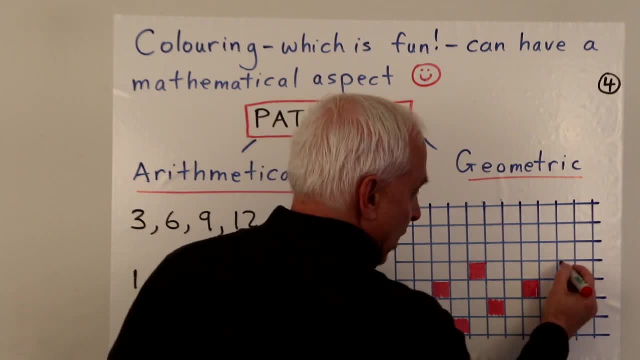 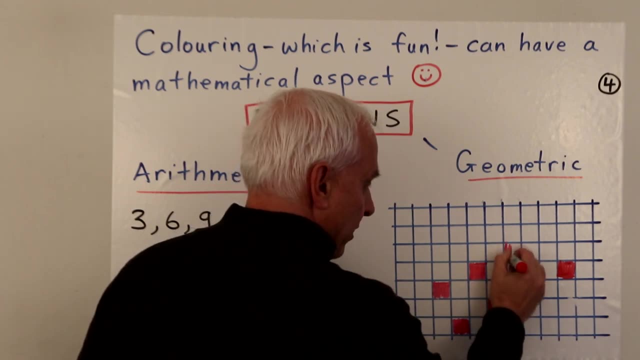 So maybe we should go over two and up one and we should colour this one. OK, so let me do that. OK, And maybe we should go over two and up one from this one and colour that one. And now let's pause. 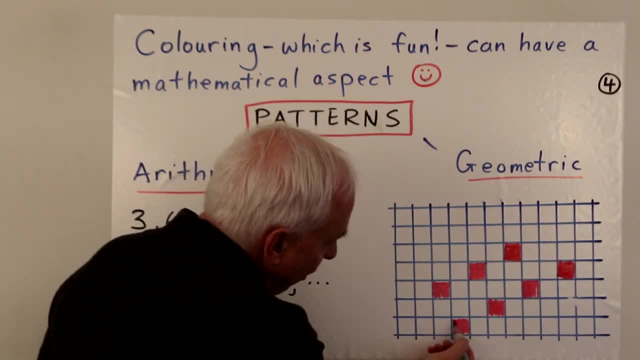 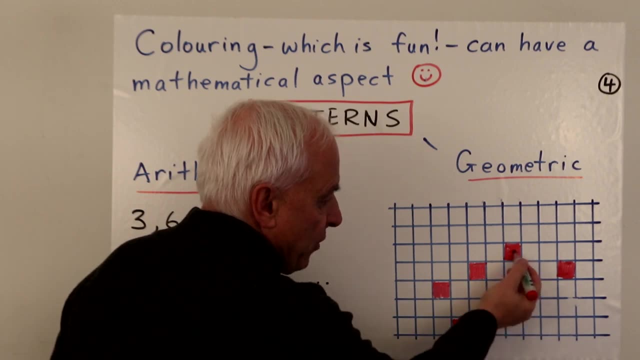 Is that still regular? Well, actually, that is still quite regular, because there's also a two-one ratio between the relation between this one and this one, and then between this one and this one, And now we've established a further such relation here as well. 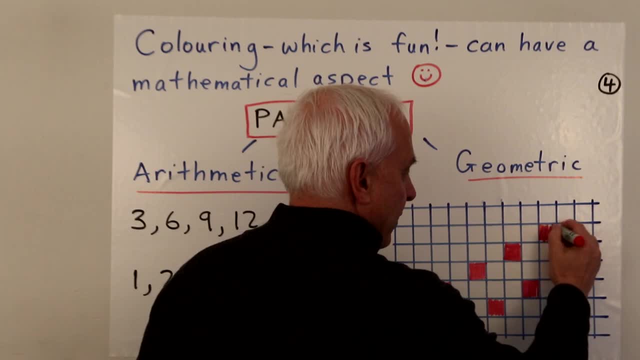 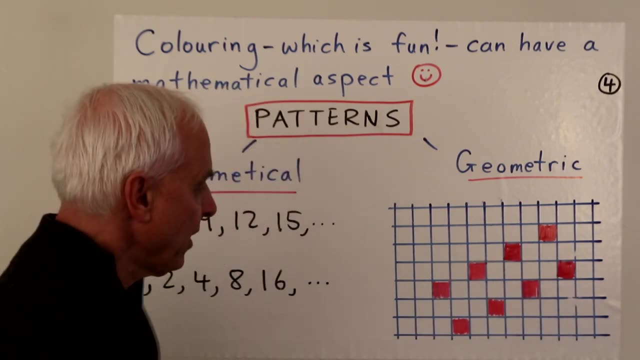 So the next one should be this one here perhaps. See, that's kind of consistent in two ways. It's sort of consistent in this direction. It's also kind of consistent with the pattern here, And maybe these patterns can be extended. 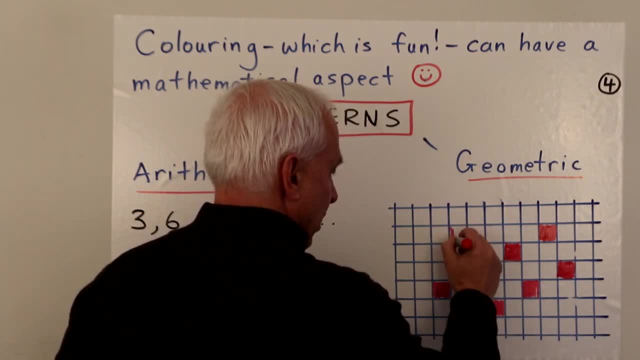 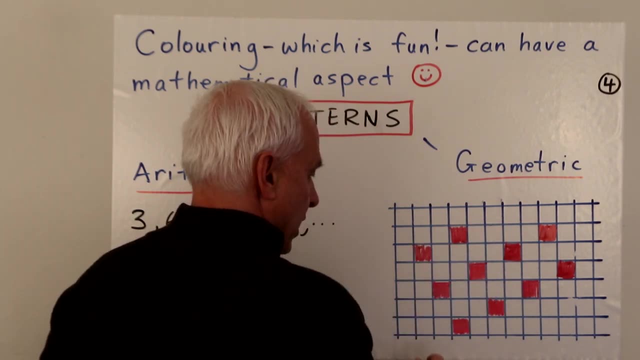 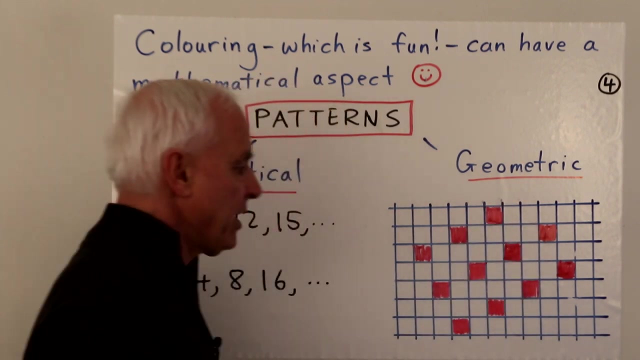 So up two and over one, up two over one. Maybe we should colour that one And up two over one. Maybe we should colour that one And up two over one, Maybe that one. OK, And you can kind of see we could also keep going down here. 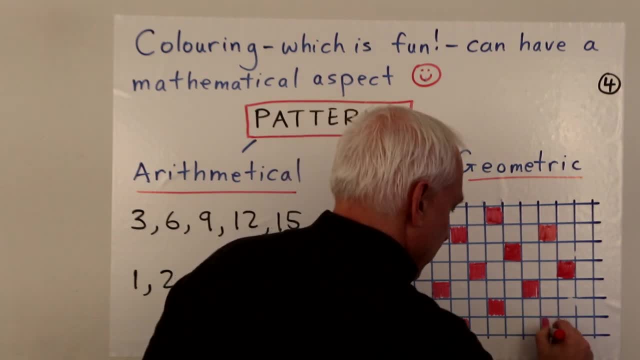 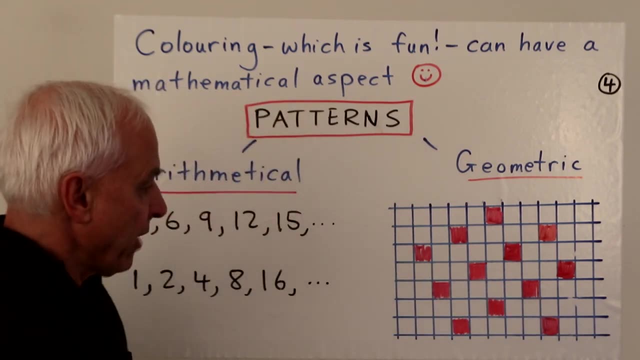 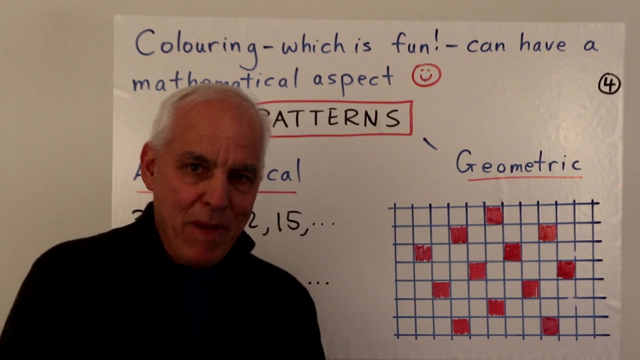 So we could go from here to here to down here. OK, So we could extend this colouring And then when you sit back and look at it, I think you'll agree that this is a pleasant kind of regular pattern. It's not quite as regular as the checkerboard pattern. 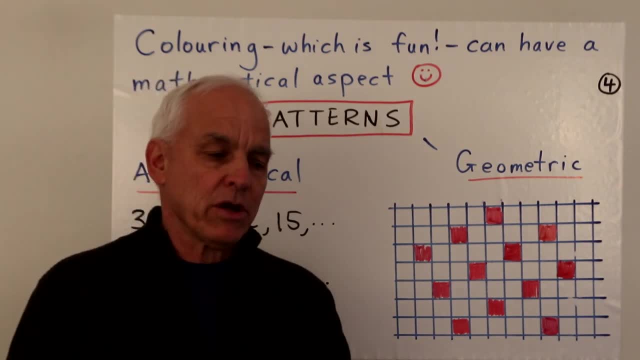 And discussing its symmetries is an interesting question. But to really do that properly we'll have to wait till we've understood the other kinds of symmetries to translation symmetry and rotation symmetry, And then we'll be able to more meaningfully discuss that. 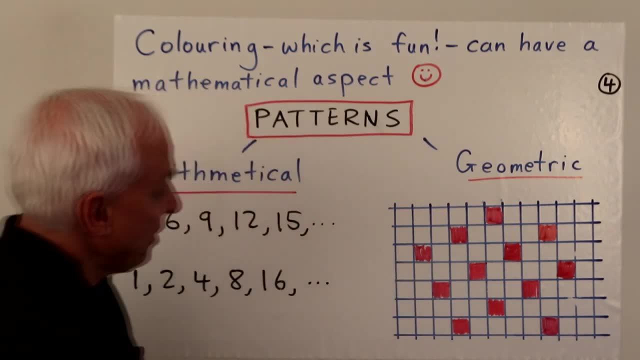 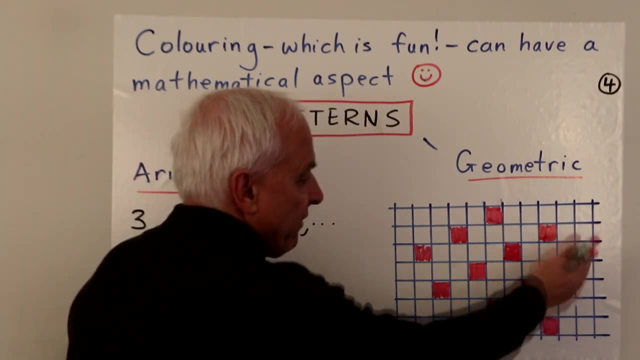 But even at this stage here we see, well, it's some kind of pleasant thing, There's a kind of a pattern And maybe you can sort of, you know, imagine students having fun sort of extending this, doing a bit of colouring. 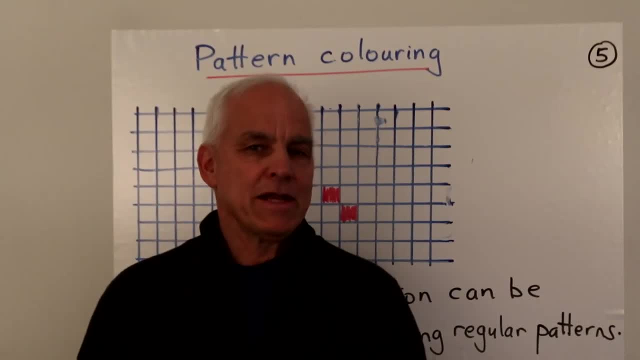 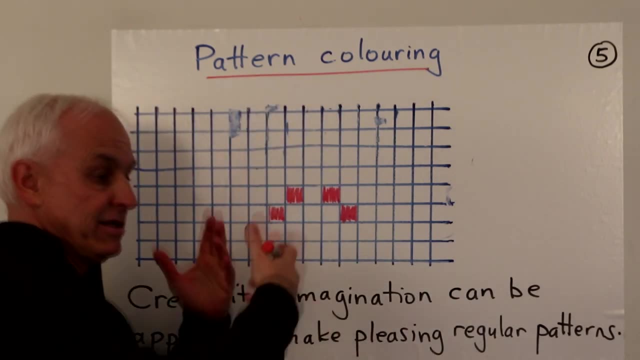 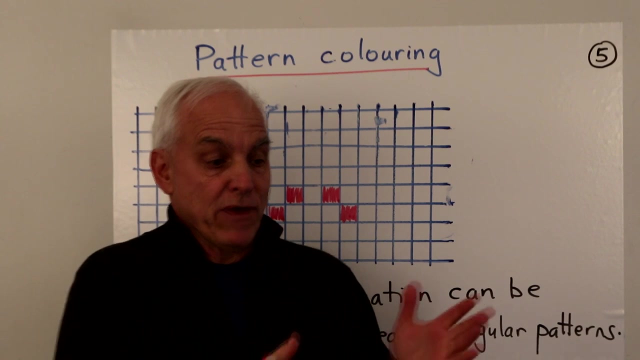 This is a very simple example. Now, I think there's a lot of opportunity here for really grabbing the attention of young people and getting them to make some nice shapes, nice diagrams, nice patterns, And we could even think about it in terms of practical terms. 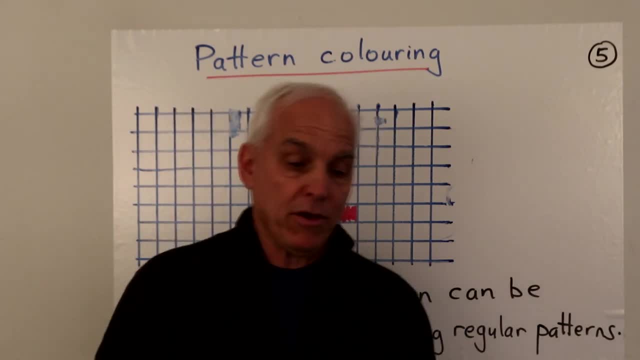 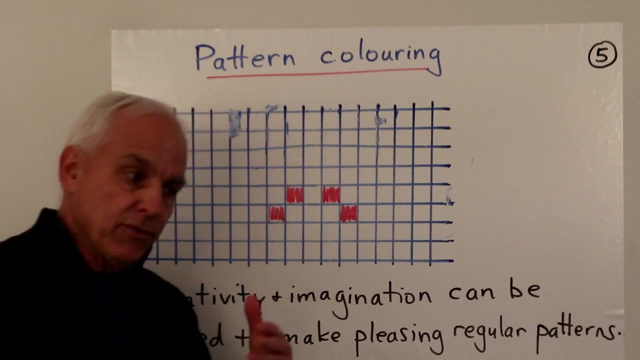 Maybe they're tiling the bathroom wall back home and they're planning out a nice pattern for the tiles so that things will look a little bit interesting. So this is a process which is involving a bit of creativity and imagination, perhaps, so students can do different things. 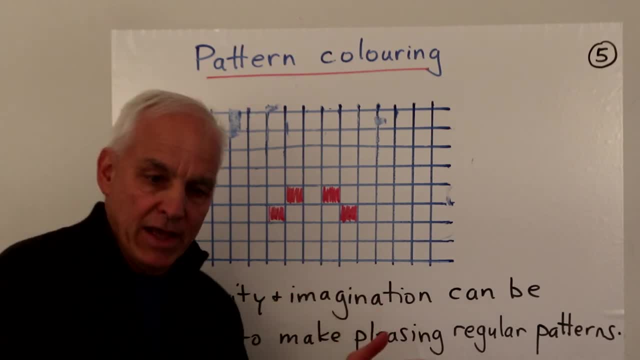 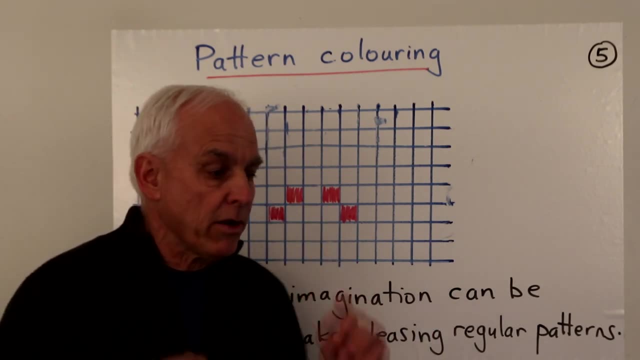 But we still want to aim towards something that's pleasing and regular. That's the critical thing. We want something that's regular so that there is a pattern. It's not just random. Okay, We're not just doing random colouring here. 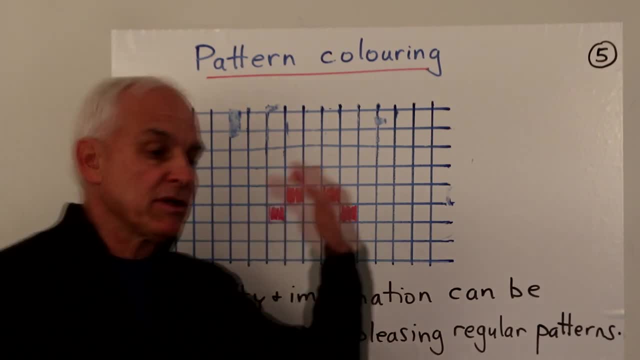 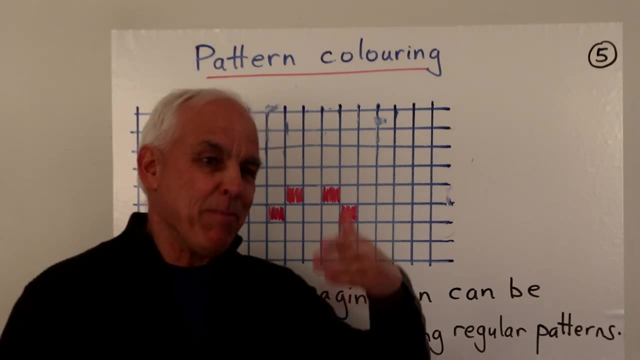 We are trying to establish a pattern, and students should be able to tell you what the pattern that they have in their minds is, And it may not always be so easy for them to implement that pattern, and practice is required. So let's do an example. 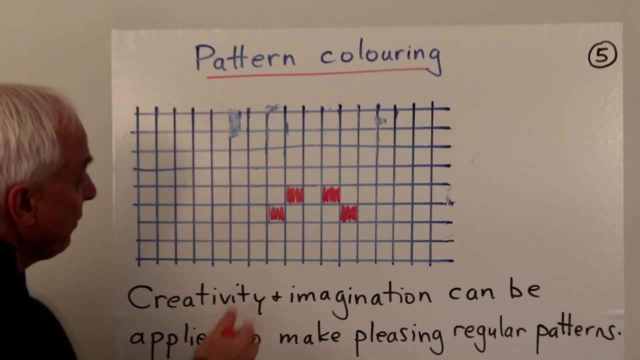 So here again is a graph paper square tiling, and we've got four tiles that we're sort of starting with. okay, We want to start with a pattern that has that as a part of it, And we want to extend this in some fashion. 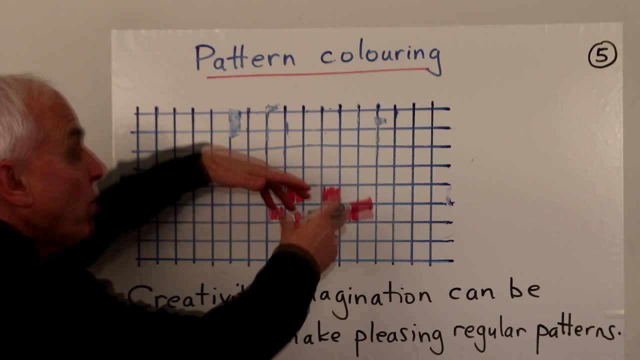 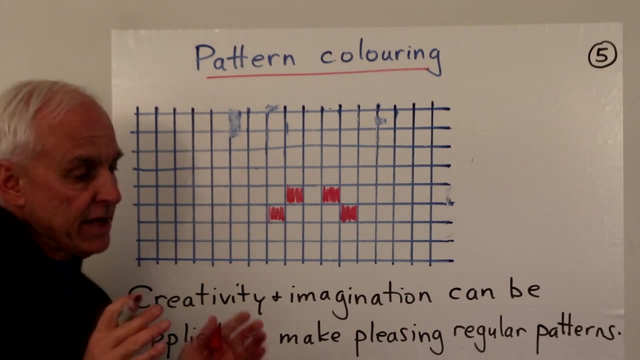 to a pleasant, regular pattern that we could, in principle, keep on extending. Okay, So there's various ways of doing this, but let's concentrate on the idea of mirror symmetry or reflection symmetry, because we've already talked about that. It's a way of reinforcing that. 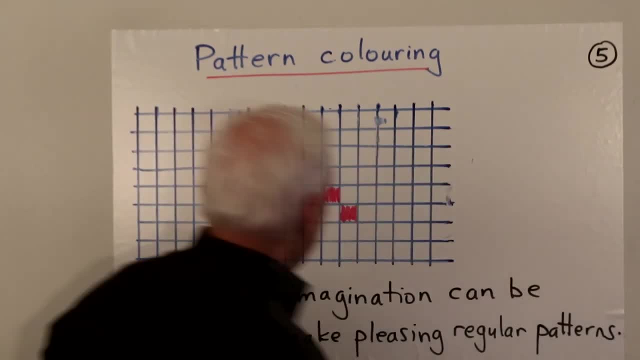 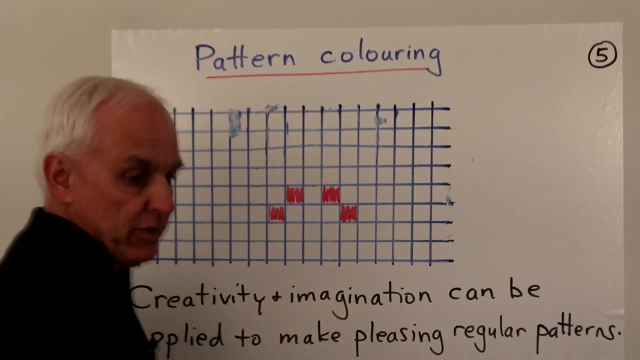 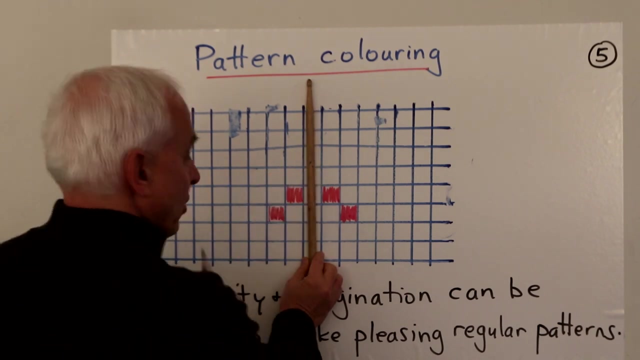 We already see that there is some symmetry here, in that the current situation is symmetrical along that axis, So a natural thing to do would be to maintain that symmetry. So whatever we're going to be doing is going to be still symmetric along here. 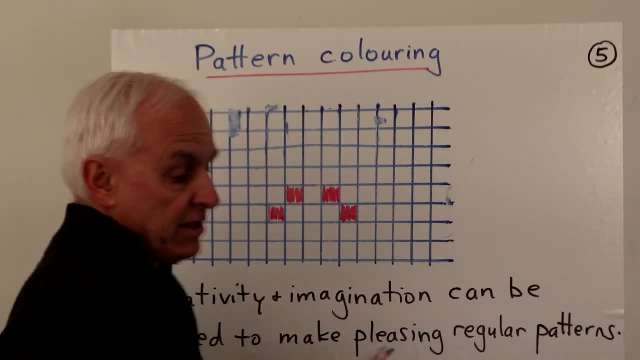 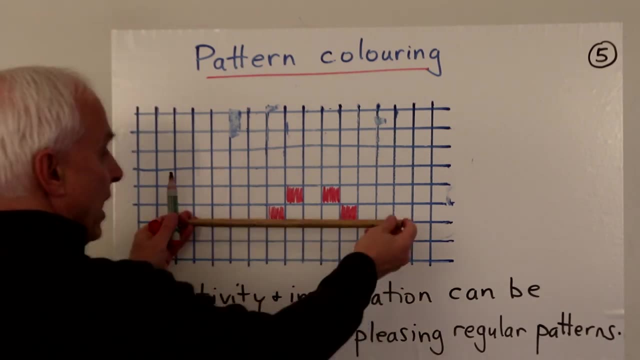 That's a decision that we're making. We don't have to do that, but that's a kind of a natural thing. Okay, So let's introduce another kind of symmetry, maybe along a horizontal axis, And we're free to choose whatever we want. 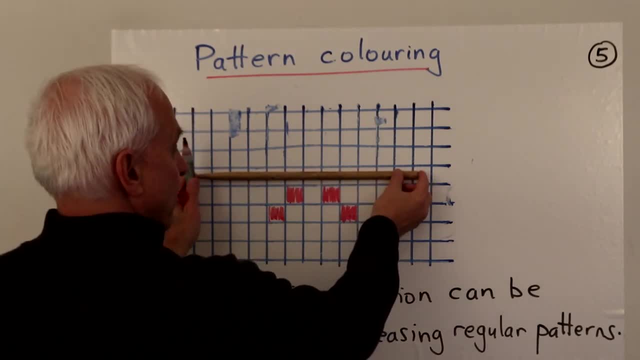 So maybe we could choose that one there. So imagine what would happen if we wanted to choose that as an axis of symmetry. So we have to put stuff on top which mirrors the stuff on the bottom. So this one will be mirrored by that one there. 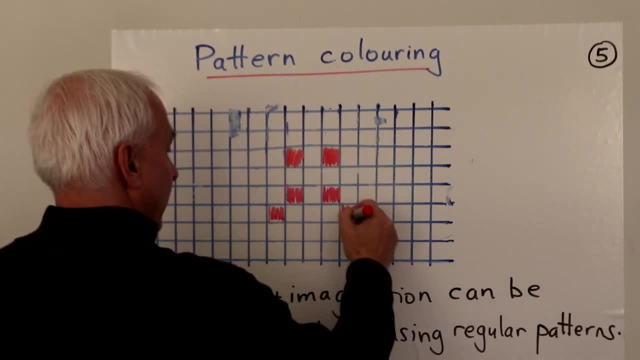 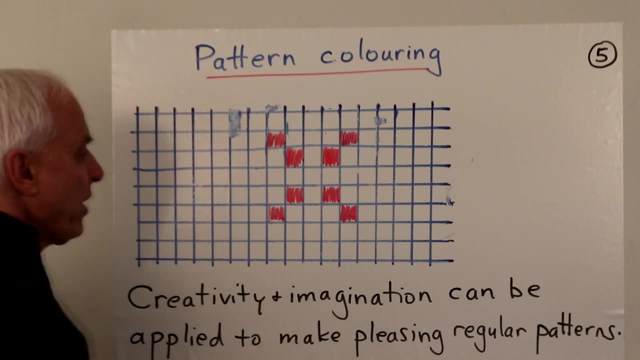 this one by that one there, and this one by that one there, and this one by that one there. Okay, great, And now what? Well, now we could- at least you know- potentially invoke some other axis of symmetry. For example, what? 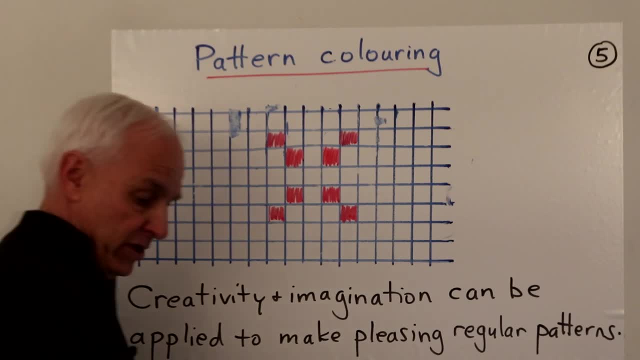 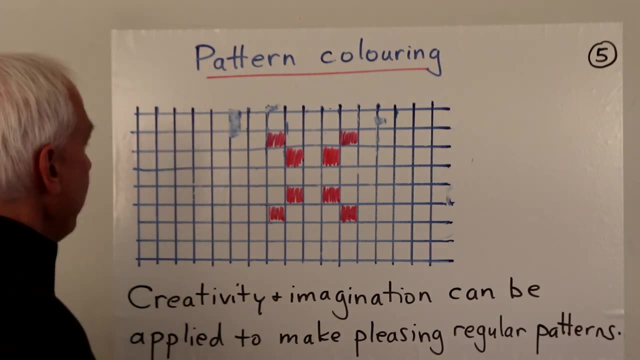 So perhaps, for example, we can have another vertical axis of symmetry. Maybe that one, Maybe that one, Maybe that one, We could choose. okay, So let's choose one. How about we choose this one? Okay, so I'm going to choose this one now. 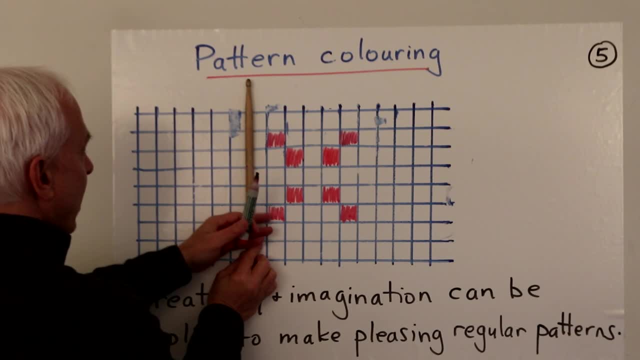 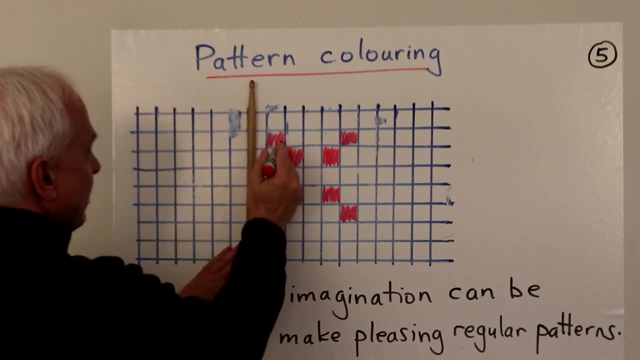 as a further axis of symmetry. Okay, so I have to just kind of copy- Maybe I'll just keep this here temporarily- I have to copy this thing, reflect it on the other side of my mind so that each one has a corresponding square. 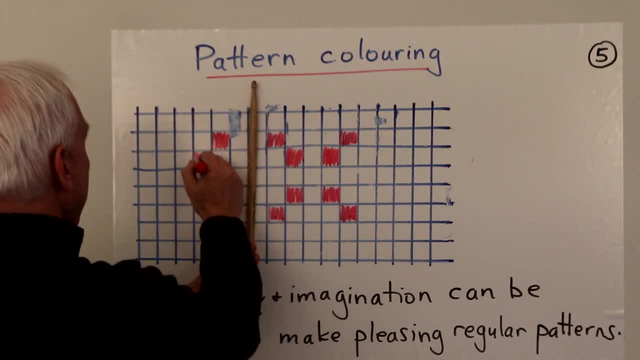 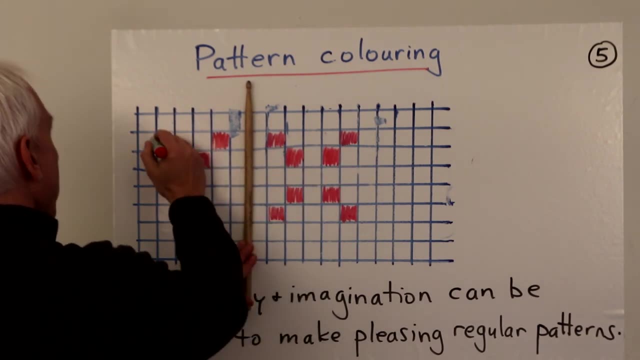 on the opposite side. Okay, let me try to do that correctly. So that one there, And now we have to do a little bit of counting. So we have to go one, two, three over and then another one. So one, two, three over. 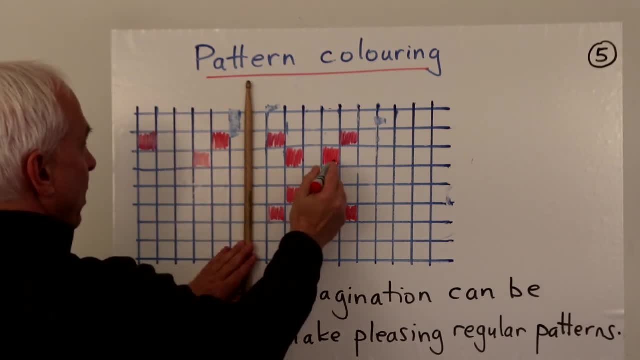 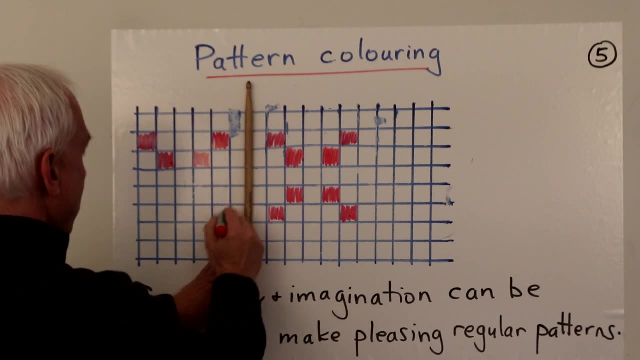 and then another one. And what about this one? Well, it'll be one in, Okay, And then we're going to do something similar with these bottom ones. So maybe like this, And then like this, And then over one and up here. 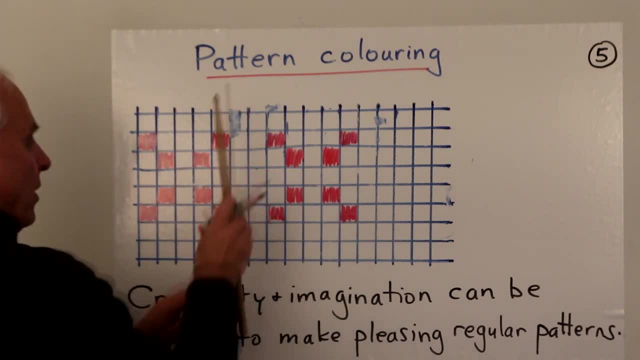 And then another one further down there. Okay, so you can see that we're starting to create a regular pattern And we could kind of keep on going, but we'd have to do a little bit of, you know, measuring and figuring out where. 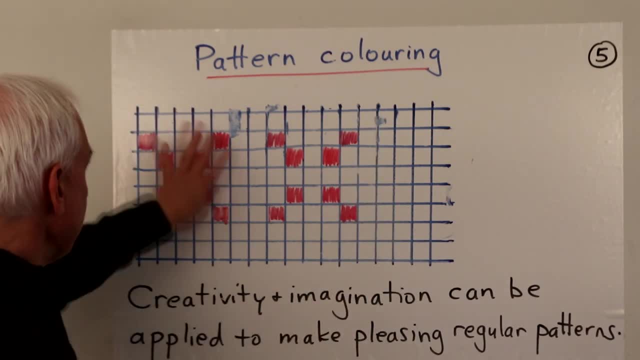 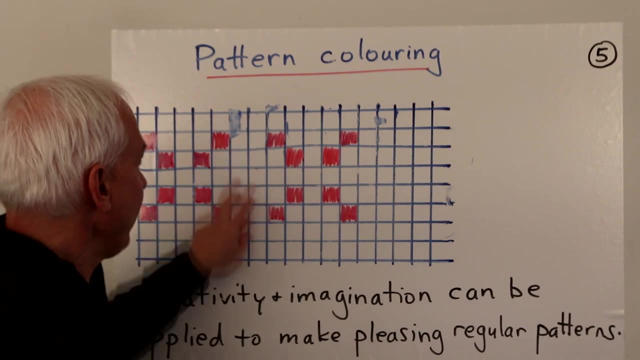 the axes of symmetry should be. So we can imagine sort of this shape here and it's being repeated here And maybe there's another copy of it adjacent over here, Also separated by two, So there might be one. let's see something like this: 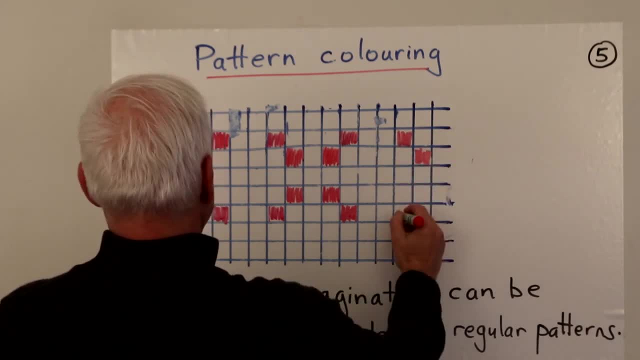 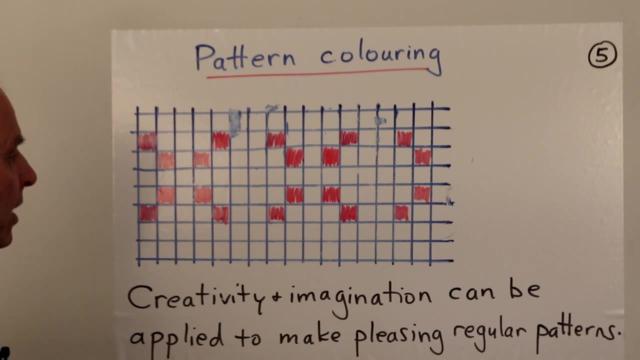 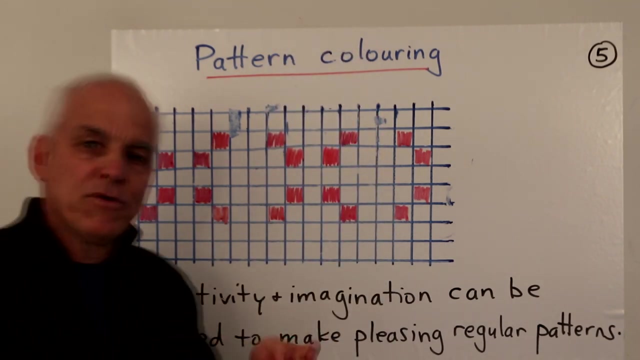 Okay, And then this, And correspondingly down here, I suppose, And over here, And then keep on going, And then we could also make further copies below and above, And then, you know again, further decisions would have to be made. 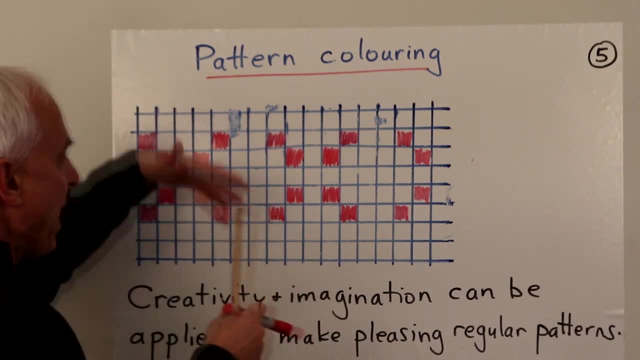 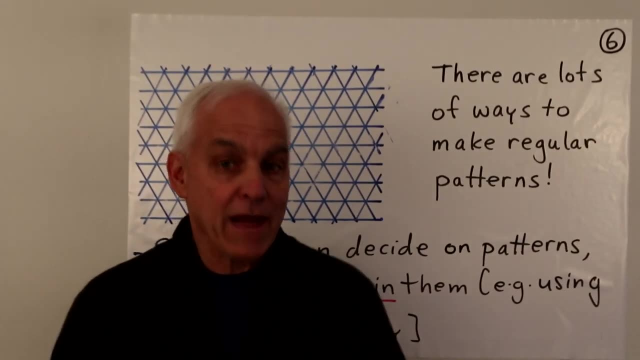 But after a certain number of these decisions, then the pattern should be clear and you know, students should be able to make a nice pattern. All right, now let's look at the triangular tiling And same kind of thing, Same kind of issues happen. 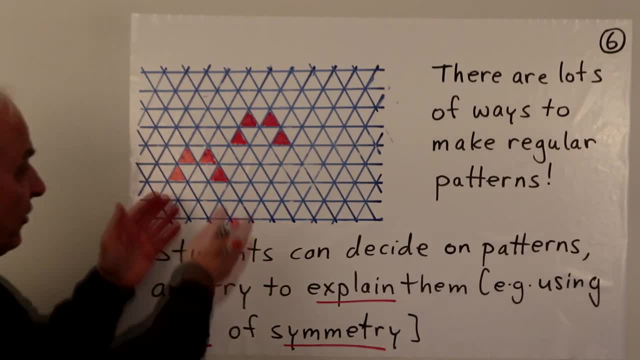 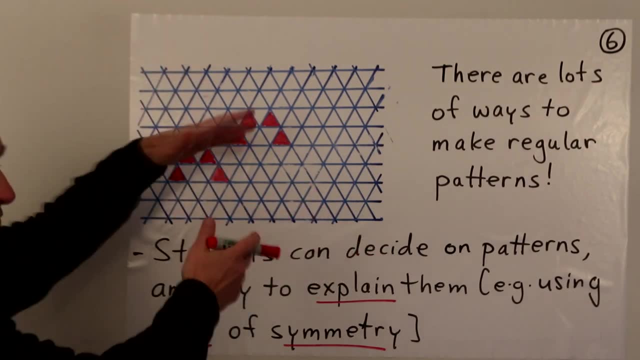 There are lots of ways to make regular patterns, even if we start with something. So maybe here's something which already has a little bit of a pattern in it, And we might want to try to extend this in some way to a regular pattern on the plane. 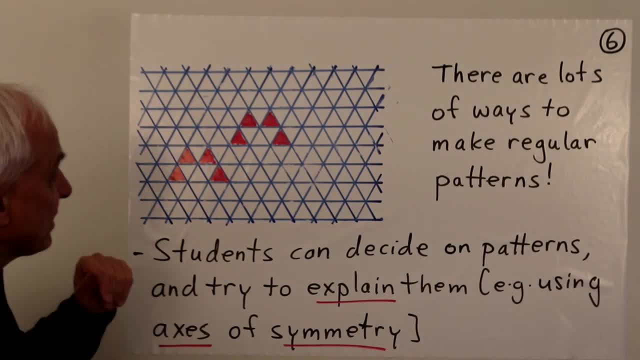 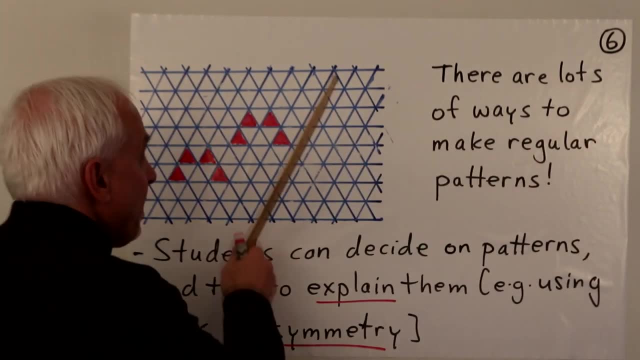 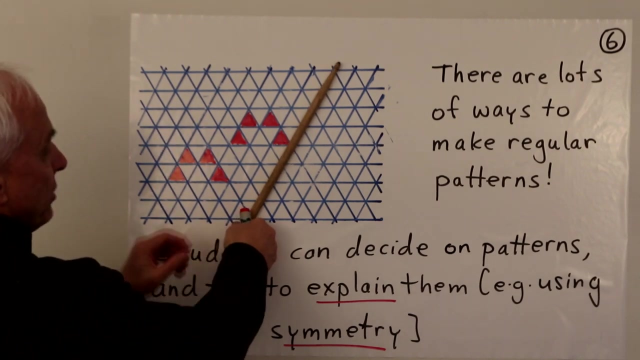 And again, there's lots of different ways of doing this, Maybe in this case, here I'll illustrate the idea of using a non-vertical or horizontal axis of symmetry. So, for example, maybe this one here. okay, How about that one? 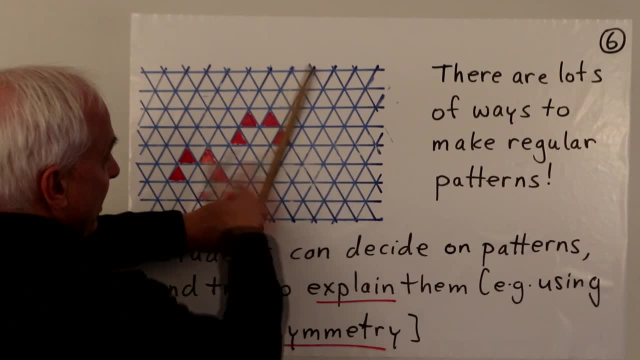 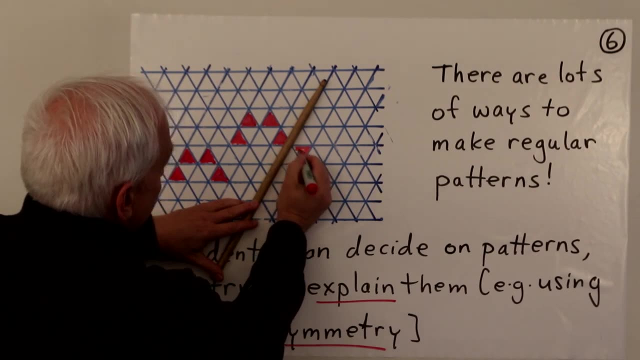 So we're going to use this as an axis of symmetry, So we want to reflect everything that we have already in this line here. So this triangle here is the easiest one. It gets reflected, So that one there And then its top corner, here is one over from. 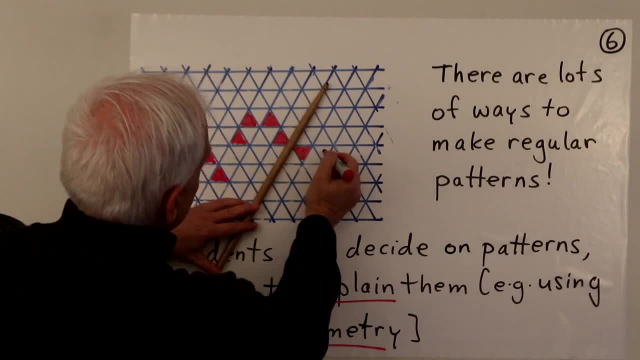 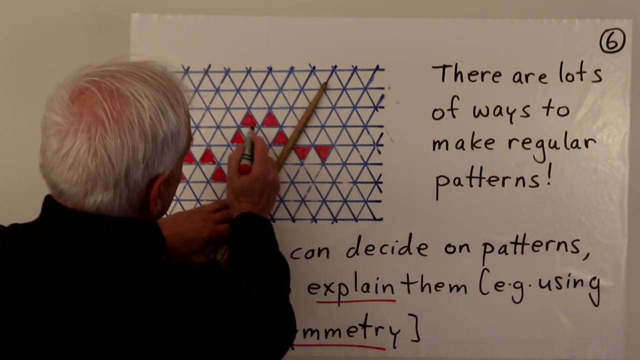 I guess that one there. Do this a little bit carefully, Yeah, I think that's the right one, Look at it the right way And then over here, this one here gets reflected. You have to sort of figure out where is it? 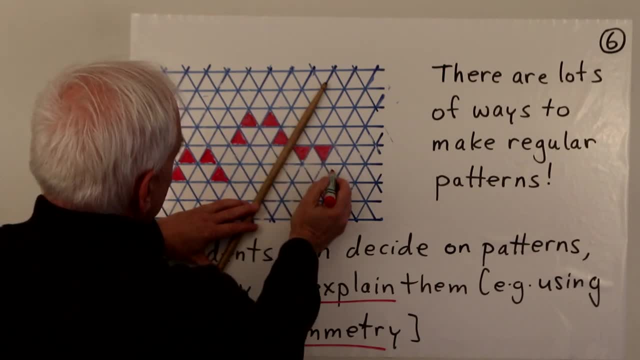 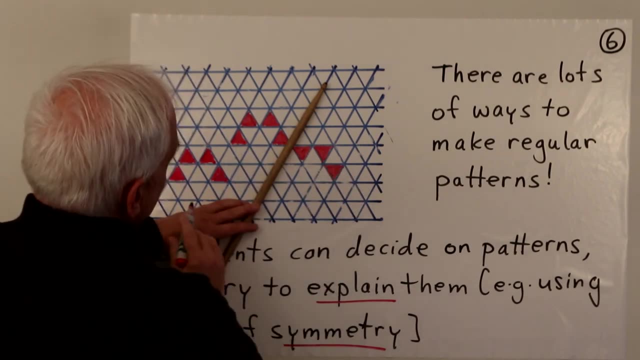 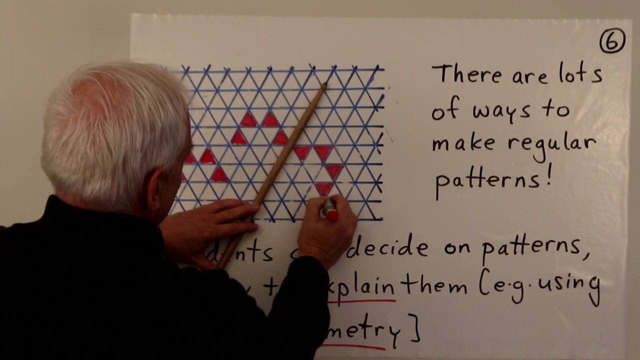 So maybe we're going one two over that direction. So one two, That would be that one there And then this one here would be sort of symmetrically, that one there. perhaps It gets a little bit tricky, Easy to make a mistake. 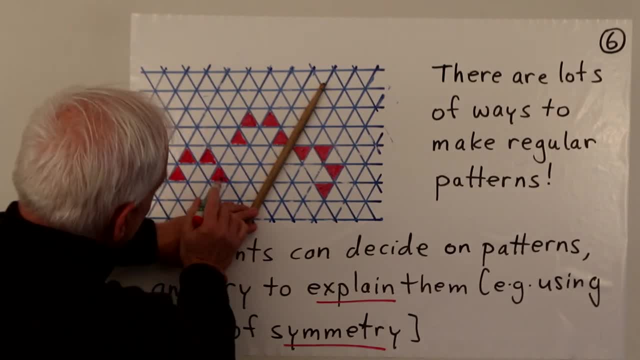 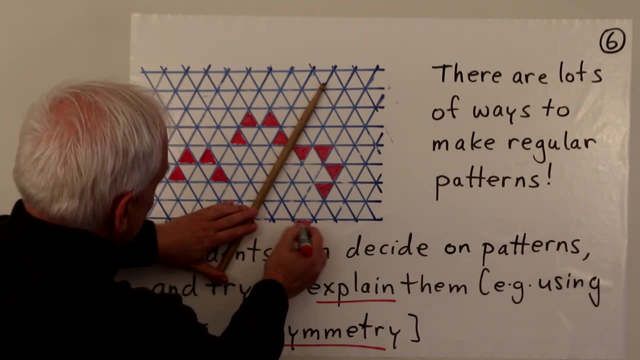 And what about down here? Do we experience anything? Probably, most of it's too far away. So two over there, So maybe this one down here would be the first one And the rest of it would be further down here. So that would be one sort of thing that we could do. 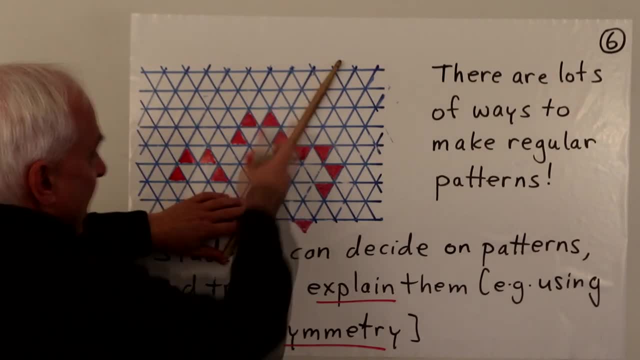 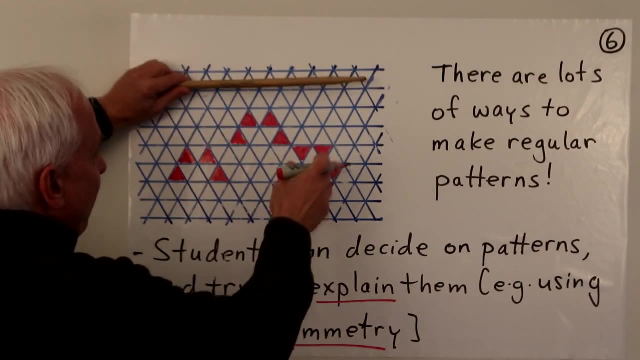 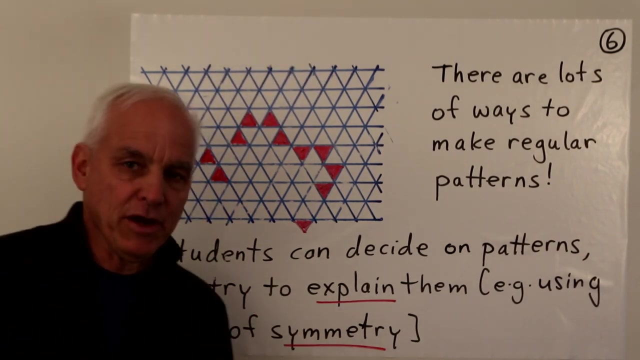 We could say that we're going to make a pattern that has this as an axis of symmetry, But that's not enough To get a regular pattern. we need to have some further symmetry so that we can keep on extending what we have. So there's lots of opportunities for creativity. 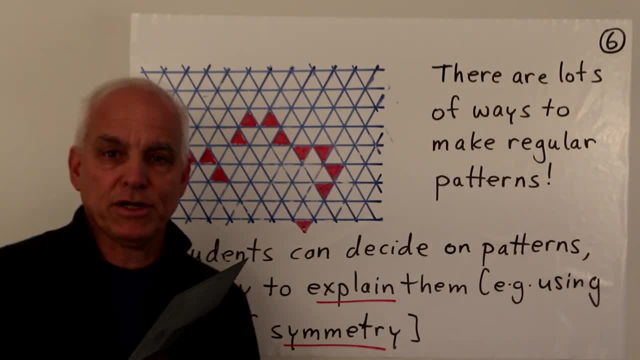 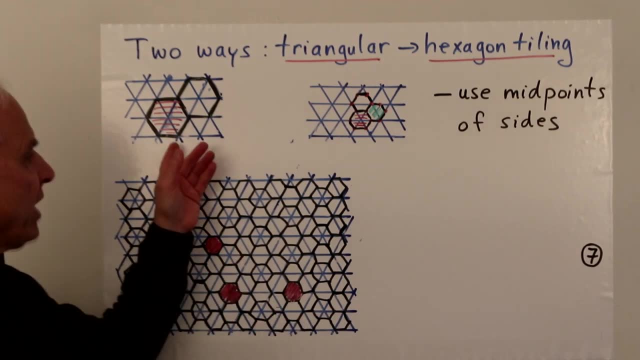 and sort of some fun pictures here. So when we get to the hexagonal tiling, we have corresponding things, Interesting questions, But a starting point is actually how to create this hexagonal tiling. So I've shown you already that you can start. 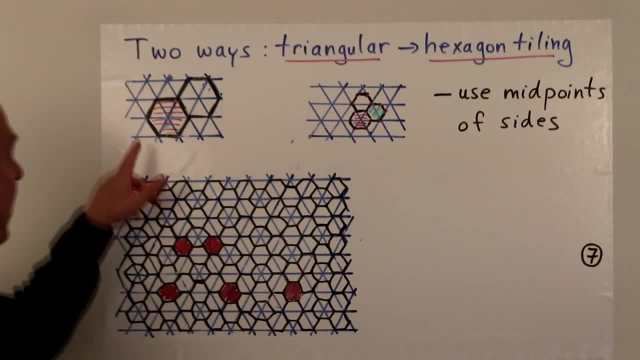 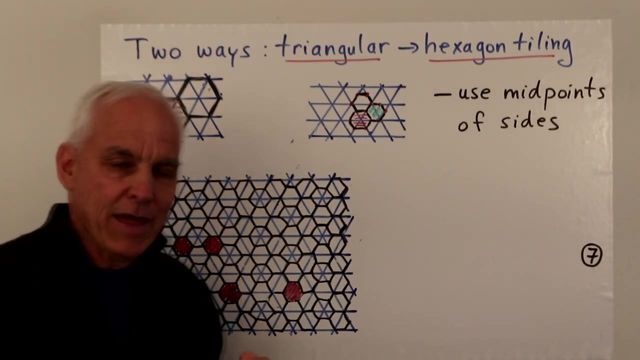 with a triangular tiling and then create these hexagons just like this, where you use the sides of the equilateral triangle as sides of the hexagon. That ends up having quite large tiles and that's maybe not always so convenient. So I just want to show you that there's a second way. 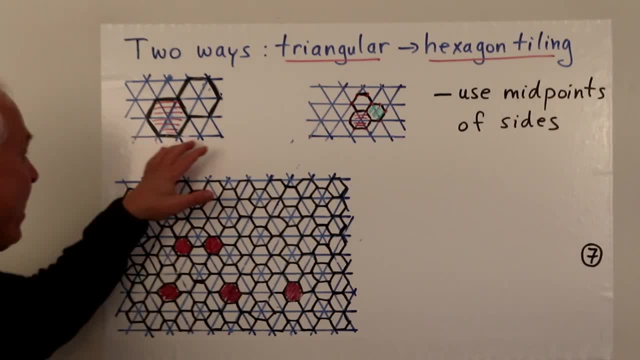 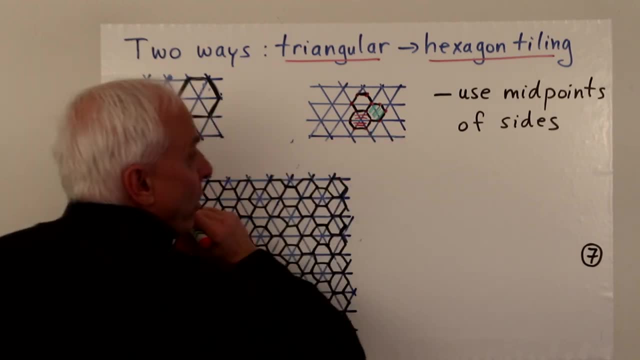 of creating a hexagonal tiling from an underlying triangular tiling, And that's obtained by looking at the triangular tiling and looking at midpoints of edges. So here's an edge, That's an edge between here and here, And I'm going to take the midpoint. 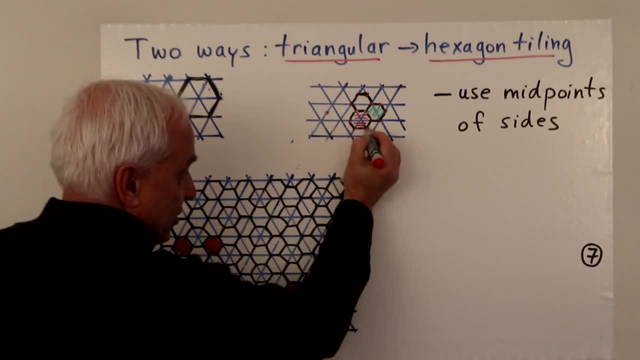 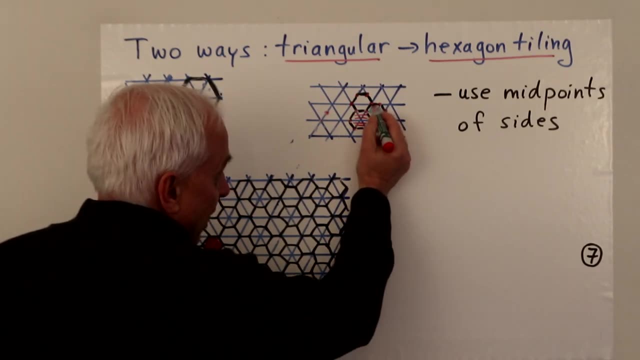 That's the midpoint. Quite a lot of midpoints here. You can create a hexagon by joining those midpoints And then adjacent to it there will be a similar kind of hexagon, but it's a little bit different. It's created from midpoints. 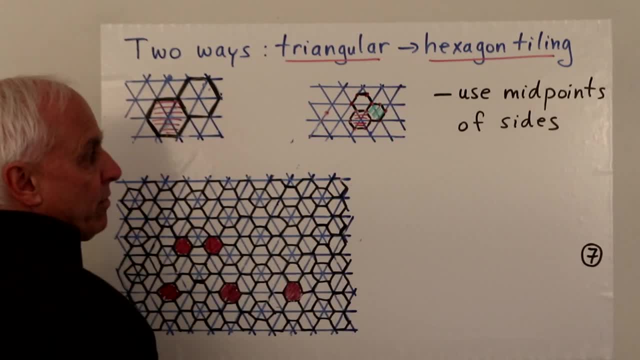 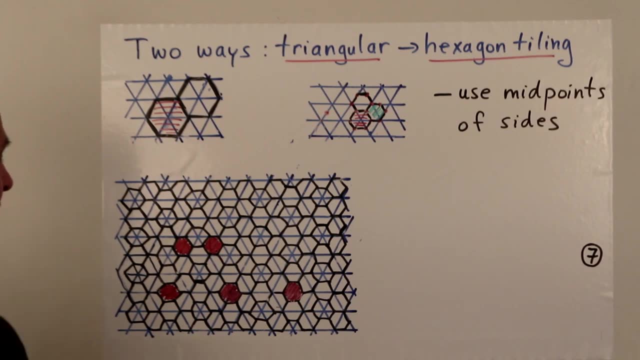 as well as vertices of the original blue thing. So you could keep on extending that. You get hexagons which are smaller than the ones over here, And I've done that over here in a somewhat more larger kind of way. So you see the underlying blue triangular tiling. 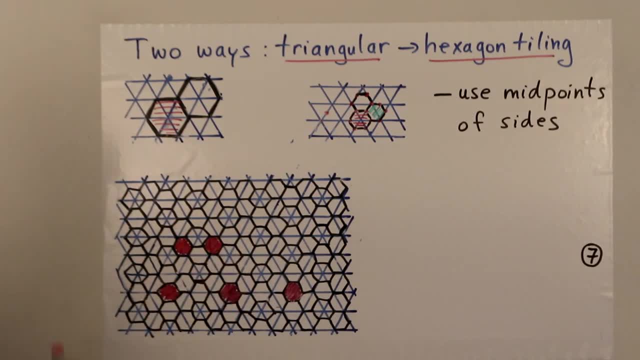 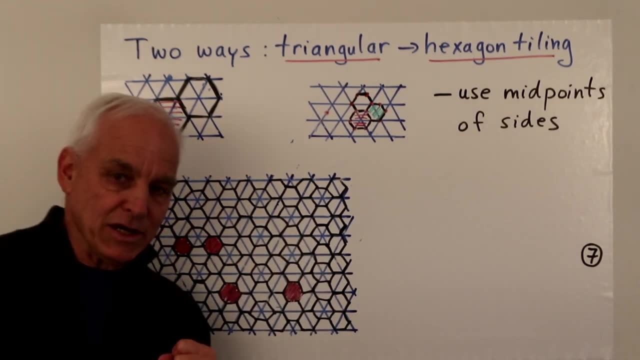 and then superimposed on it a black tiling of regular hexagons a little bit smaller than these ones here. This is a little bit more amenable to coloring issues because there's more room. Note already that this way of constructing them. 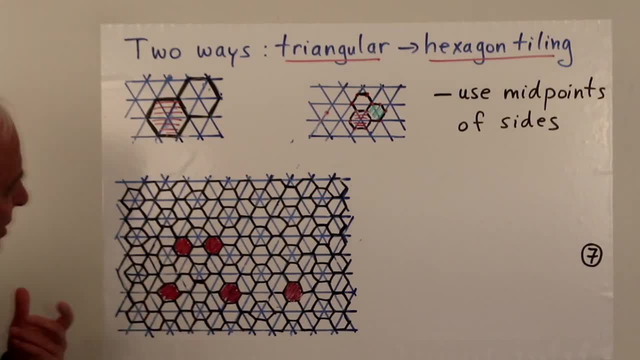 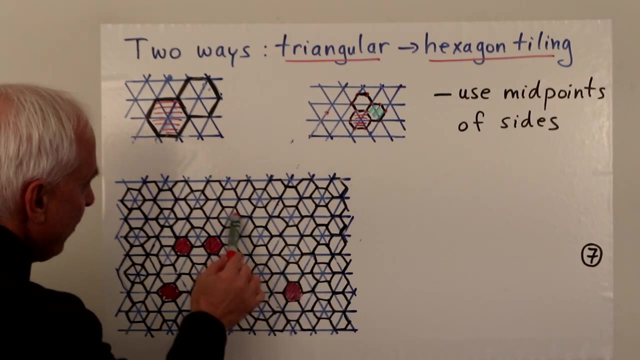 makes or brings out a certain kind of pattern. already Some of the hexagons that we've drawn have interiors which have three blue lines, For example, this one, this one, this one. There's already kind of a regular pattern for those hexagons. 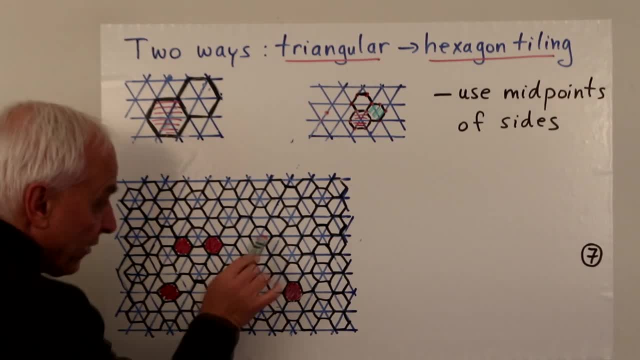 And the other ones only have a single edge through them, Like this one here only has a single edge, which happens to be in this direction, While this one here has a single edge in this direction and this one here has a single edge in this direction. 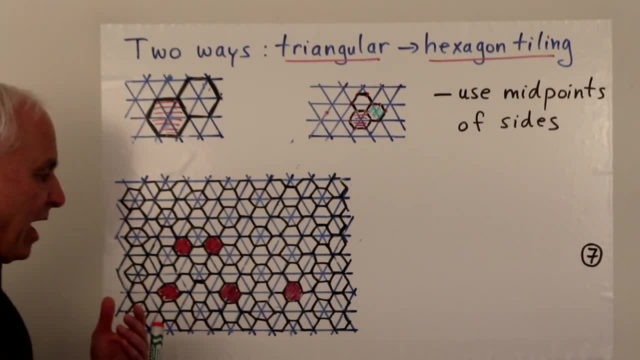 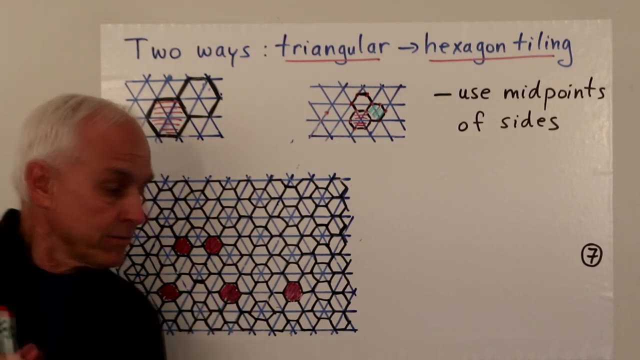 Those are the three possibilities. So the other ones are kind of divided, if you like, into three different kinds, depending on the orientation of that central line that they have passing through them. So it's already reasonably interesting Even before we've even started coloring. 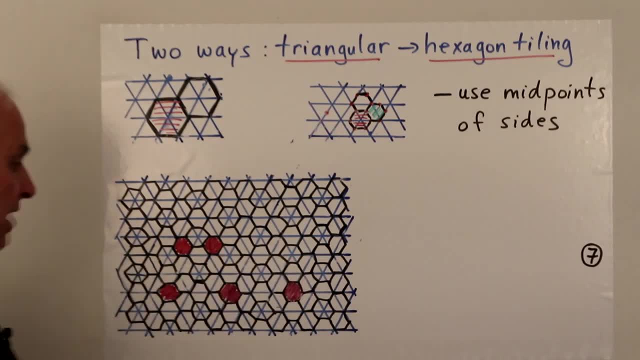 OK, but in any case, I've kind of colored some tiles. Maybe this is sort of an introductory thing. So there's some tiles And maybe we could ask students: OK, how can you extend this tiling? Maybe use some reflections. 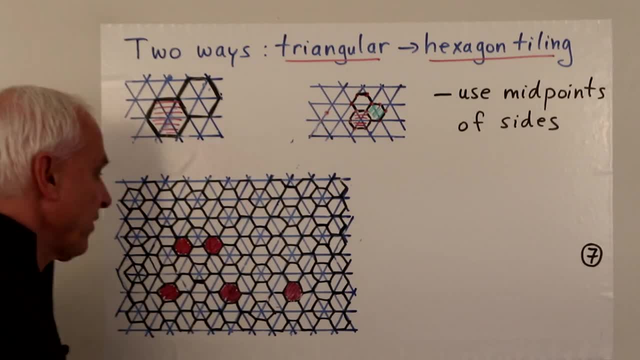 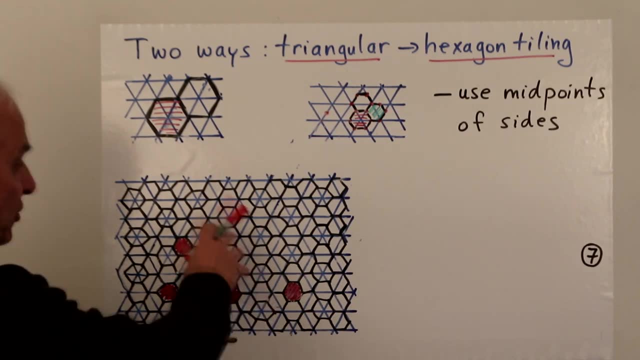 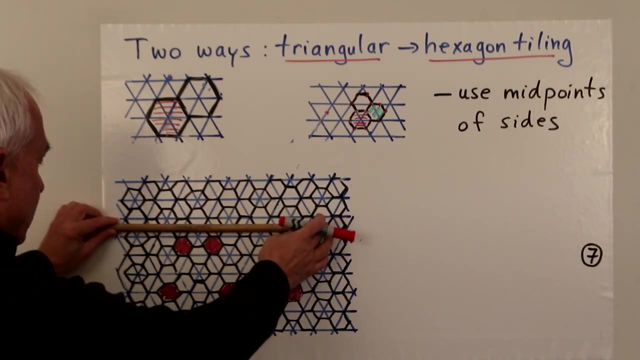 So a simple thing to do is to choose some relatively simple axis of reflection, But we want an axis that actually maps the underlying hexagons to themselves. OK, so let's say we choose. say that one there. OK, does that look reasonable? 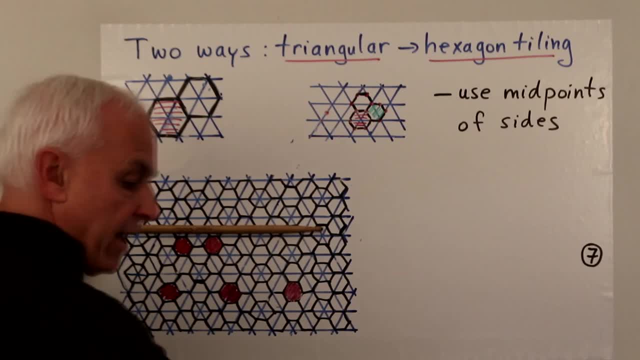 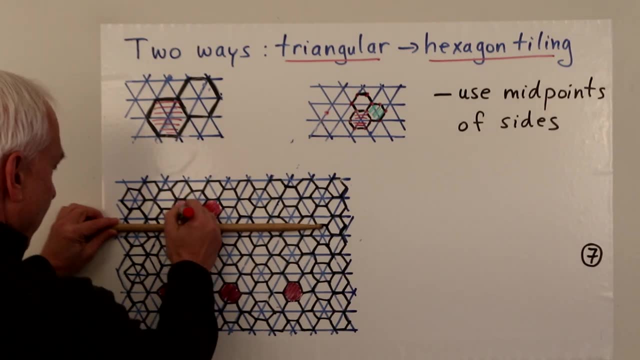 That one there. OK, so if we did that, then this thing here gets reflected up to this one here, This one here gets reflected up to this one here, This one here. so it'll be one, two, three, And we have to go one, two, three. 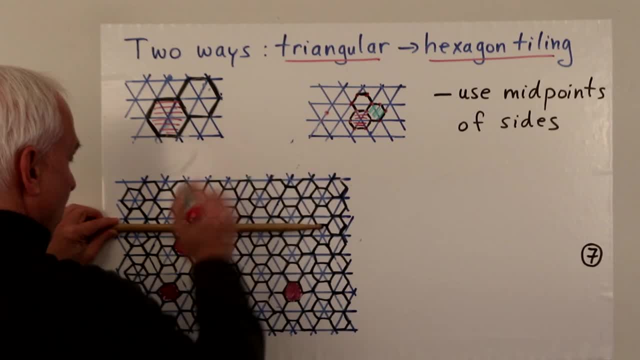 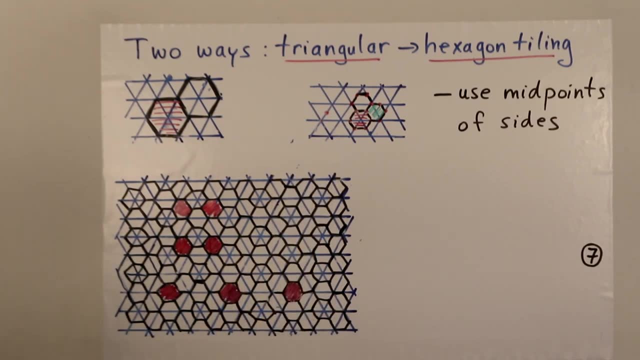 And then up here. so it'll be up here somewhere off the page. In fact, all of these other ones will be off the page. OK, what about another kind of axis of symmetry? Well, you know, it's more complicated. 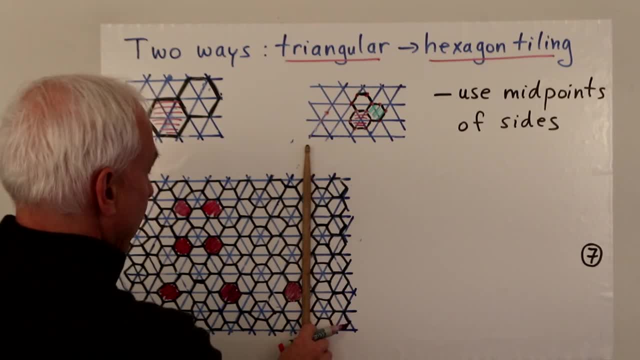 We could take a vertical axis of symmetry and say, like this one here, OK. and then we could copy this one over on the other side. You know, like OK. So there's all kinds of different ways of making regular patterns. 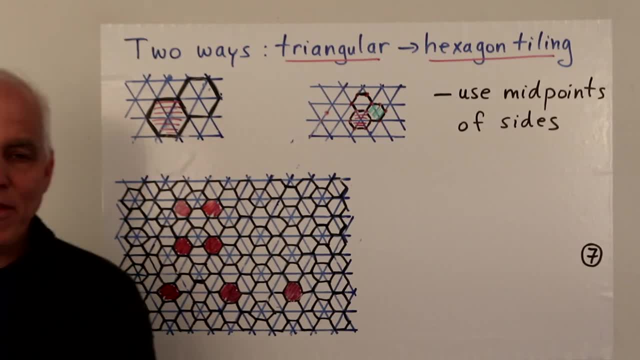 And you know, I think it's a fun thing for young children just to play around and create something that's pleasant. It gives them familiarity with these tessellations so they become comfortable with them And they become sort of tools that in their minds 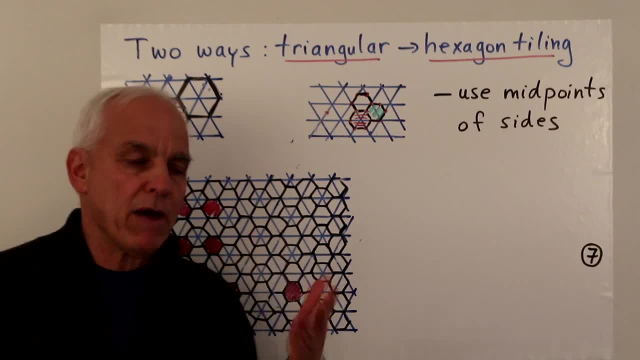 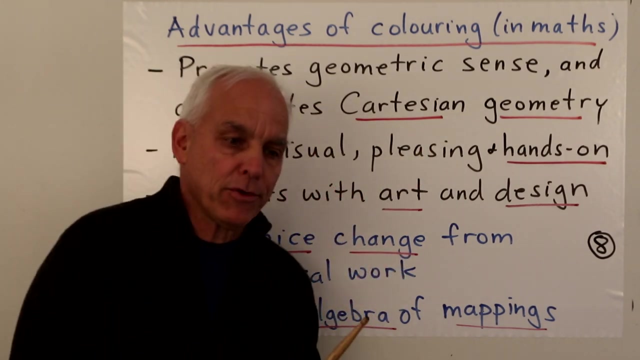 they can use these later on for various things. They know about them. They have a bit of understanding of the geometry of these tilings and of the basic shapes. OK, so to summarize, what are the advantages of this kind of approach to teaching young children coloring or patterns? 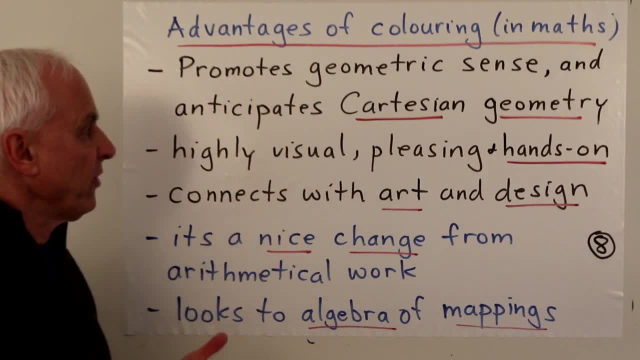 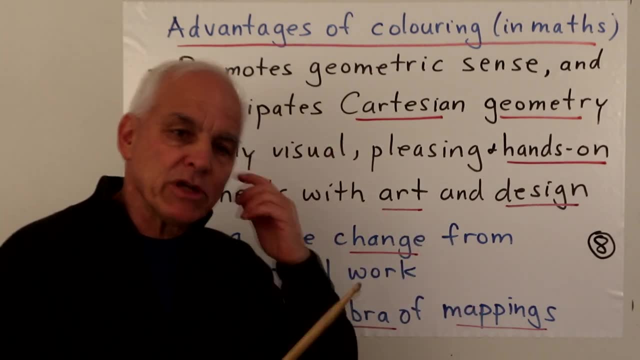 in mathematics. Well, I think, first of all it promotes geometrical sense And it also anticipates Cartesian geometry. So once we start doing Cartesian geometry a little bit later, our familiarity with the square lattice and the other two will be of very good use. 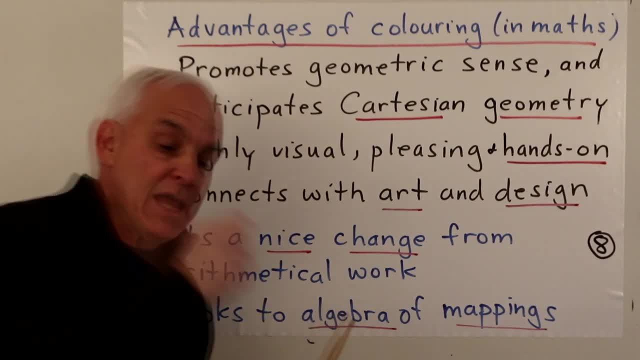 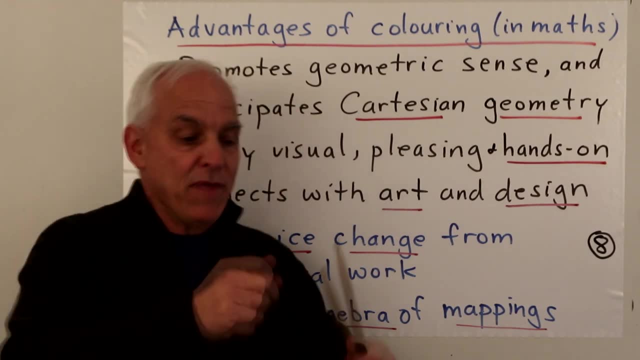 It's highly visual, It's pleasing And it's hands-on, So it's something that kids can actually do. You can get them away from their screens, put stuff in their hands. They can actually do something OK, And it's not just arithmetical calculations. 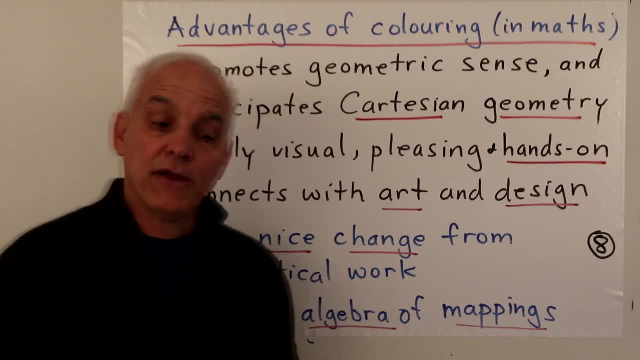 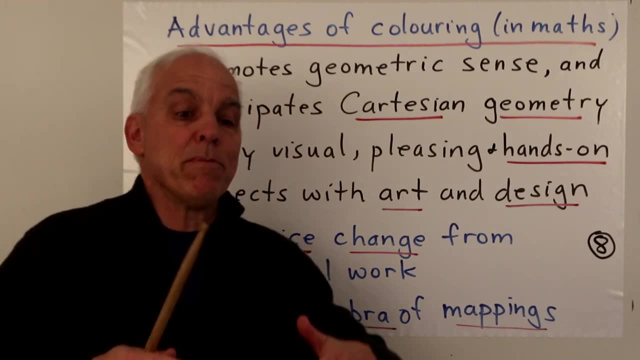 So it naturally connects with art and design. It's going to appeal to those students with an artistic bent And of course, it's a nice change from arithmetical work so that we balance what students are doing and not just doing arithmetic all the time. 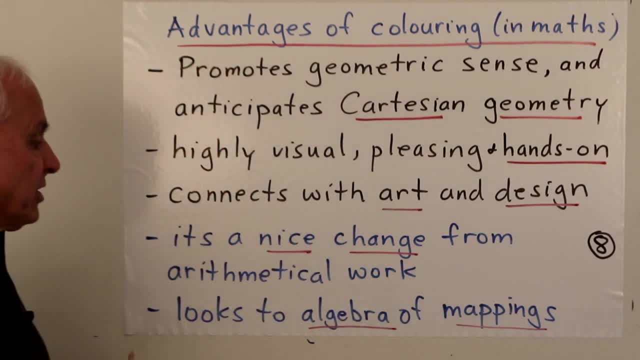 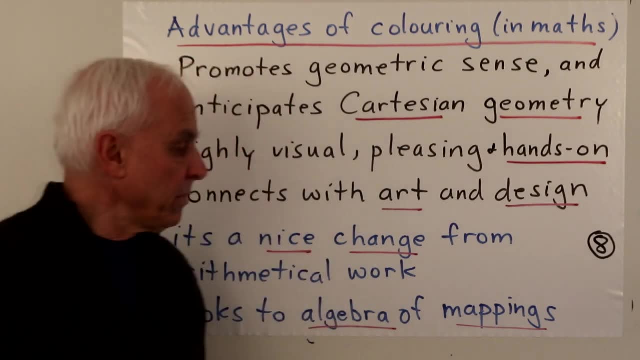 They're doing other things, And this is the geometrical side which is very important, And also it kind of looks forward to the algebra of mappings. So in our next we will be talking about not just reflection symmetry but also translation symmetry. 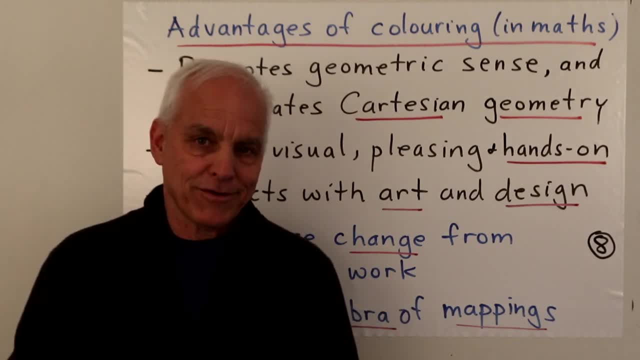 still more or less in the context of these regular tilings. I hope you'll join me for that. I'm Noah Wahlberger. Thanks for listening. 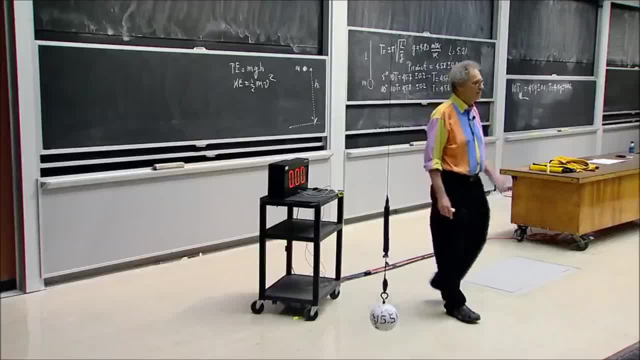 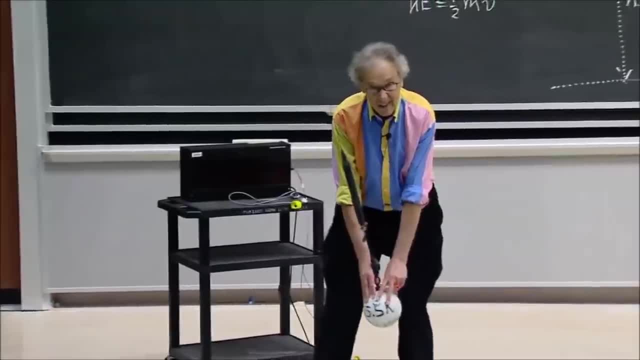 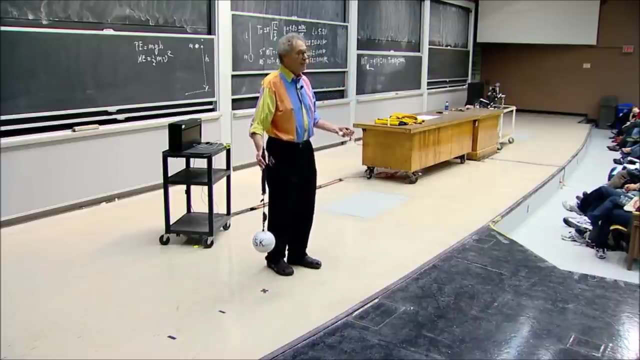 Because energy we believe is conserved. So if you bring a pendulum at a certain distance above the ground, like this, and you let it swing, when it comes back here it is almost exactly at that same height. It cannot be higher. That would be a violation of the conservation. 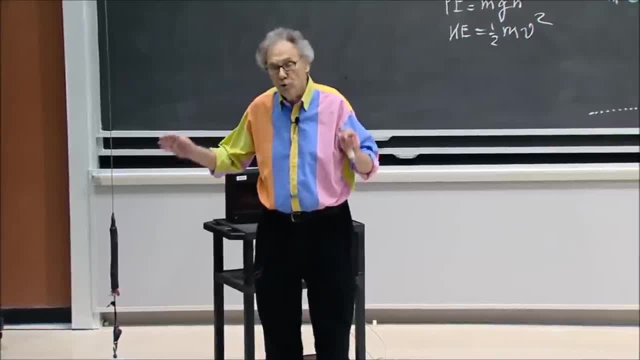 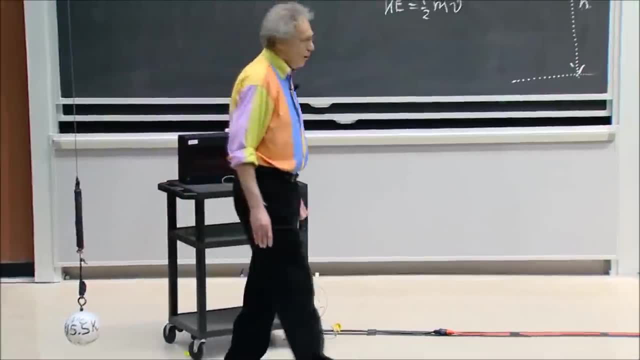 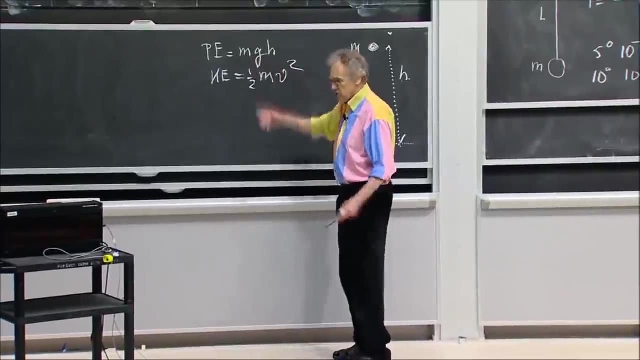 of energy, But since the air drag is so small, there is almost no damping. And this whole idea is behind demolishing buildings. With a building demolishing, you take a huge mass, you lift it up over a distance, h, and then you put your target, which is your house or 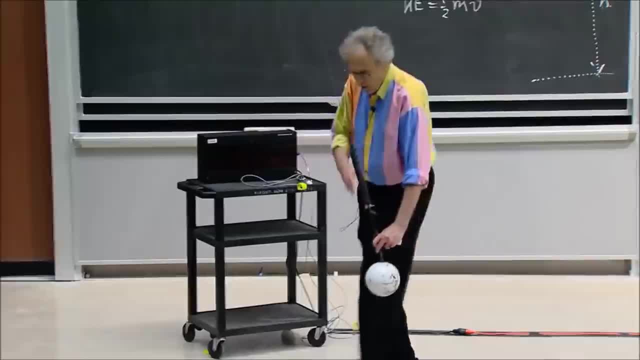 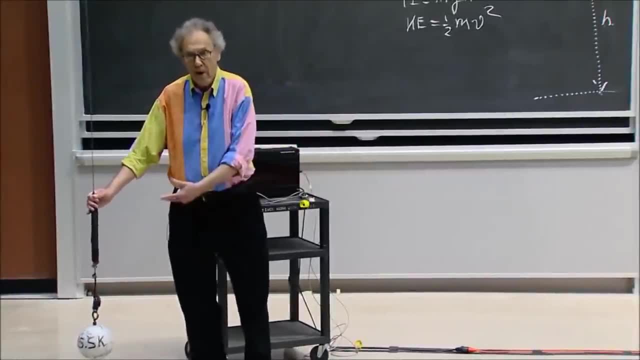 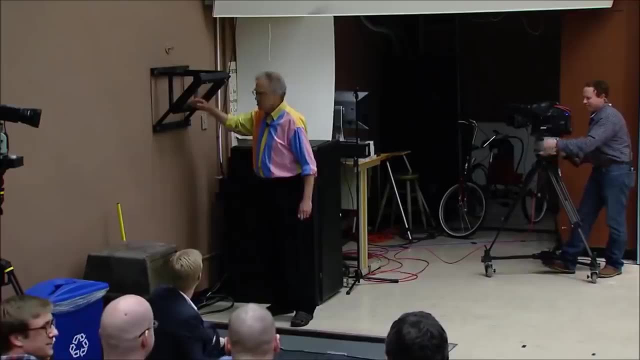 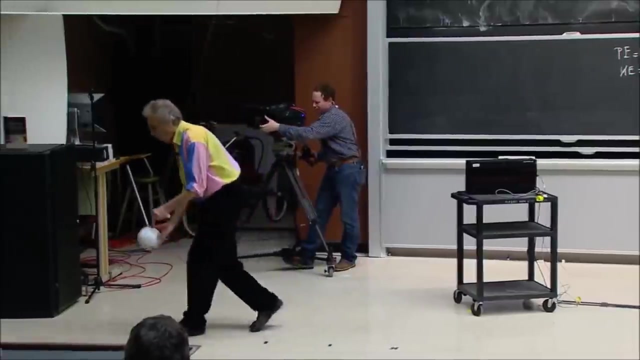 whatever it is right at the bottom when all this potential energy is being converted to kinetic energy, And so this object is hit with an enormous amount of energy at high speed and you demolish thereby the wall. This is a glass wall, So if I bring this object exactly at that glass wall and if I'm clever, 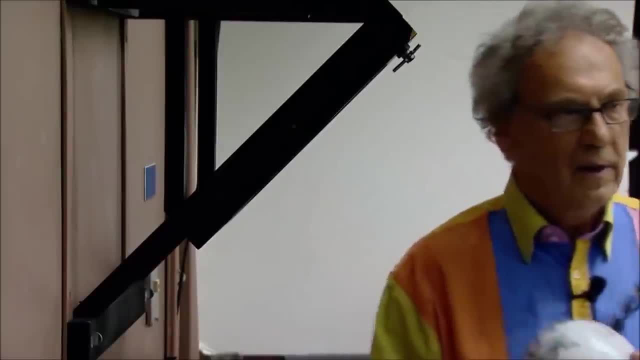 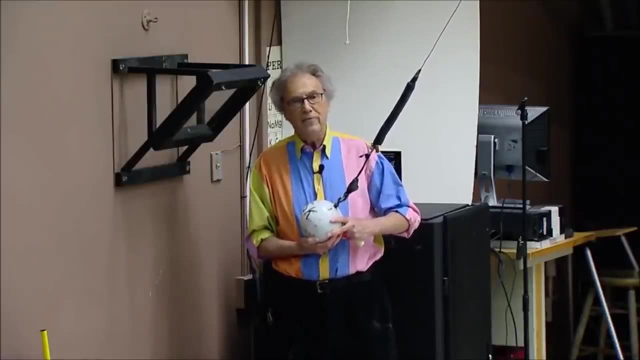 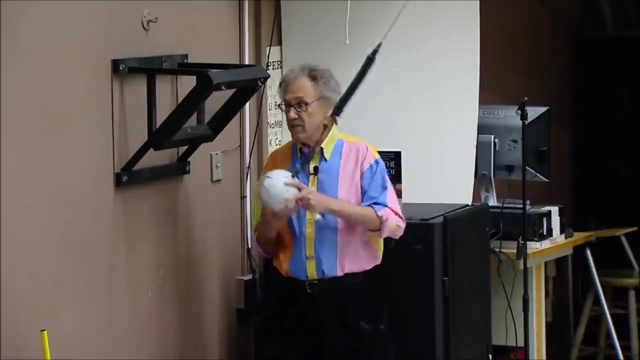 enough to let it go with zero speed. it could not break that glass. But if my hands shake a little and if I give it a little push, then of course it can't come back and it may want to go higher than this and that would mean